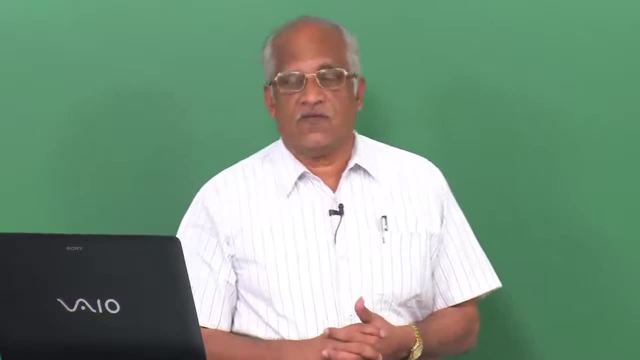 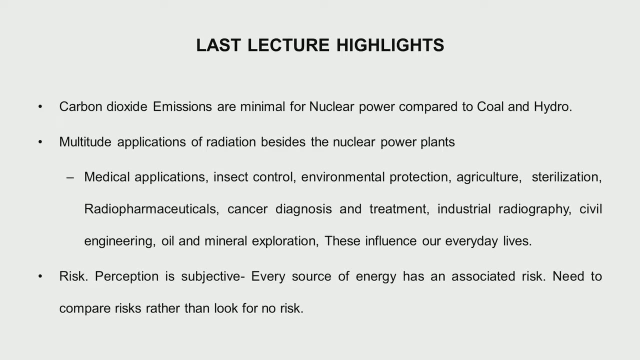 Then we went into some other aspects where the radiation utilization has been there, like in the field of medicine, In environmental protection, in agriculture, then sterilization of most of the articles used in surgery, then your gas radiopharmaceuticals and its utilization in cancer diagnosis and 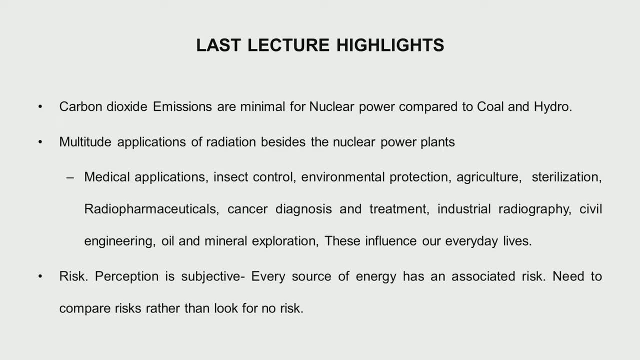 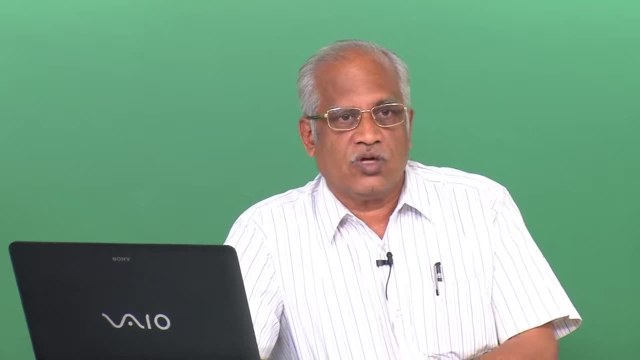 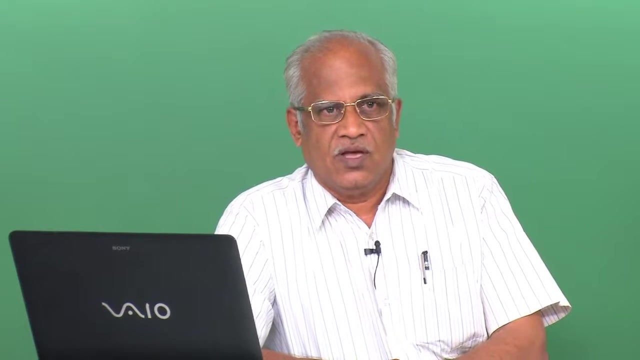 treatment, then, of course, industrial radiography, food preservation and a variety of uses which we come across. Thank you. Finally, we saw one aspect, of course: the story of three men and a tiger. I told you that there is a risk perception of everybody, but there is nothing like absolute. 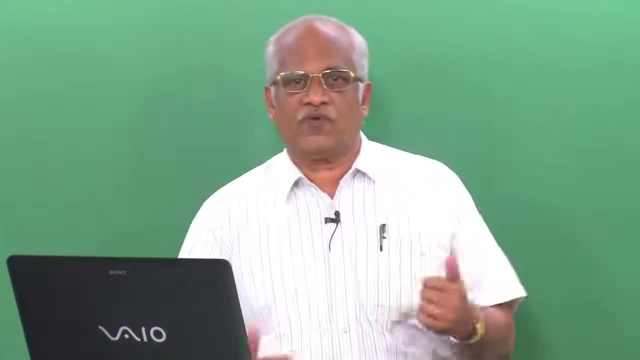 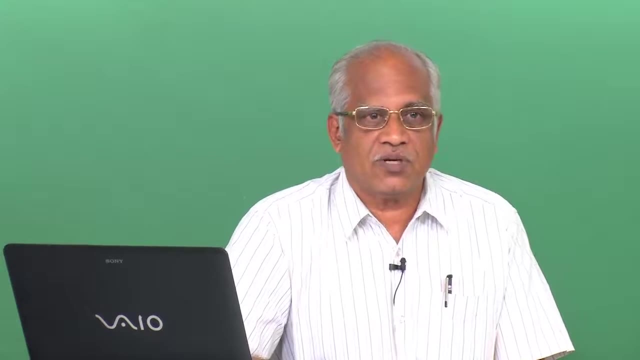 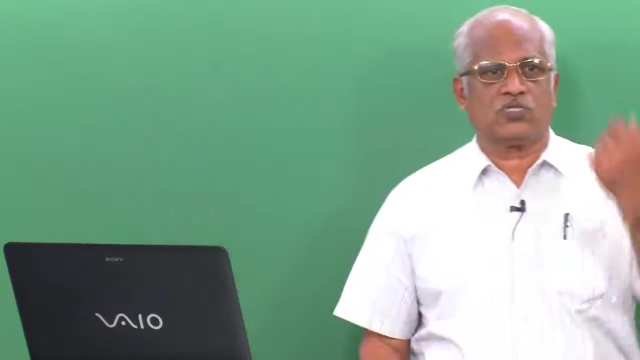 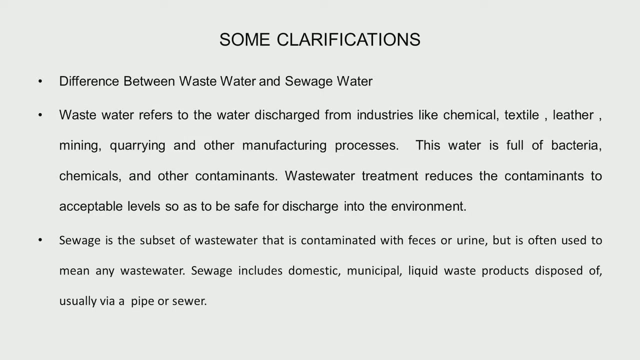 risk, zero risk. You have to compare the risks of different things and, as you know, returns, you get more when you take risks in the investment business. However, in the last lecture I got some questions from some of the students. One was: I talked about treatment of wastewater and treatment of sewage water. 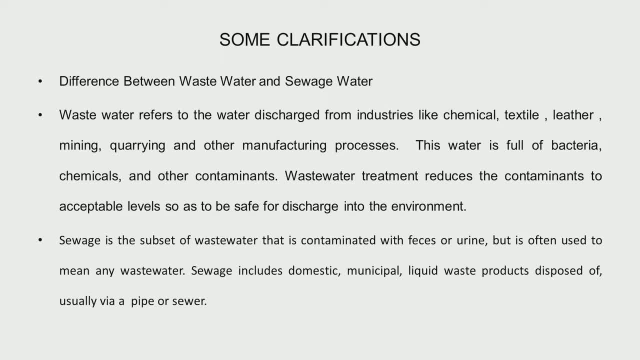 So the question was: what is the difference between the two? Wastewater refers to the water that is discharged from the industries, like chemical industries could be leather industry, textile industry, mining or any other manufacturing process industry- and this water contains lot of bacteria, chemicals and quite good number of contaminants. 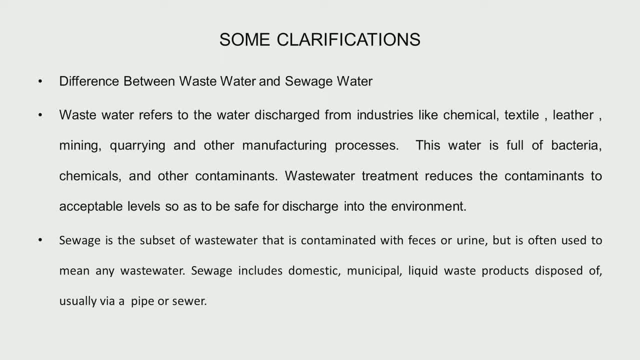 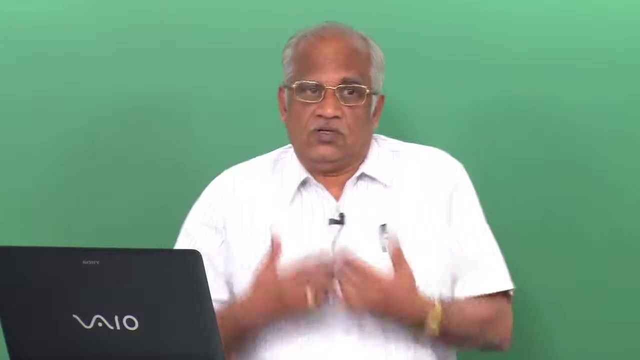 and when you do treatment with radiation, it reduces the level of the contaminants to acceptable level. then you can discharge it to the environment, whereas the sewage water is that water Which is contaminated with the human fixes, the urine, and not only which is harmful it. 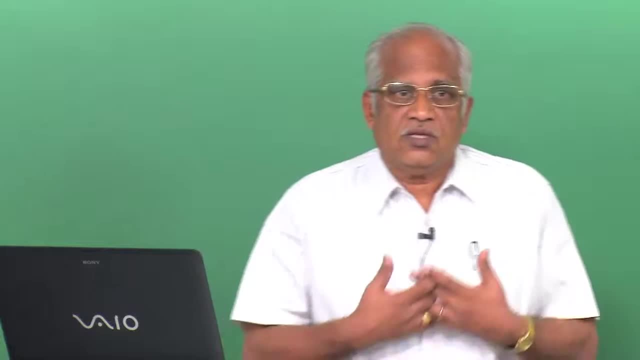 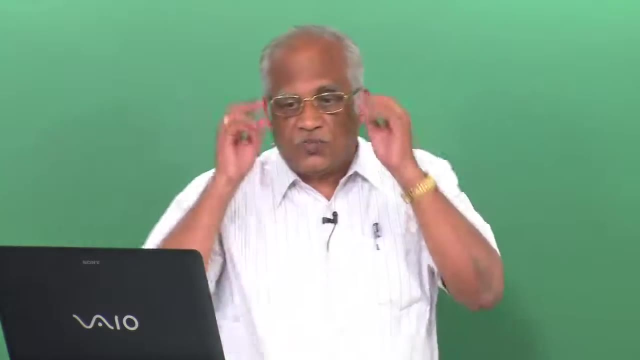 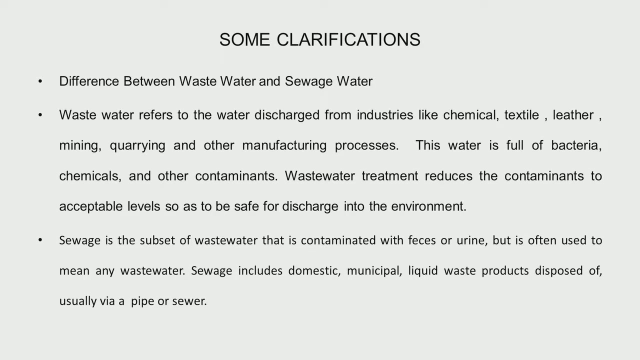 contains a lot of pathogens, lot of bacteria. So essentially it includes domestic waste, the municipal waste and waste products which are disposed of usually through a sewer pipes. So that is why the name sewage. So this, I hope, clarifies the difference. 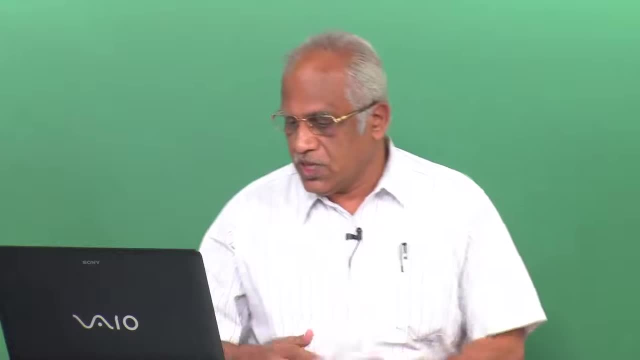 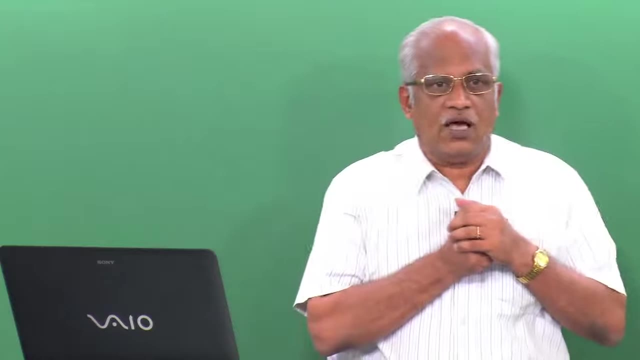 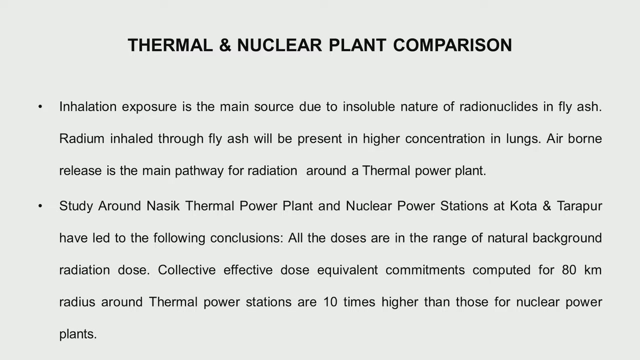 Thank you. The difference between the sewage water and the wastewater. Now there is one more clarification asked, talking about the radioactive releases from the thermal and nuclear power plants. I had made a mention that coal contains thorium and uranium. when you dig it out and this gets. 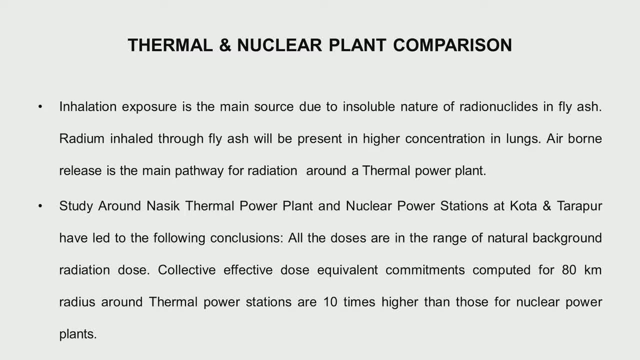 released when you burn it, It also gets discharged, It also gets to the fly bash, etc. So basically, how does this get into our system? This release is basically due to the radionuclides in the fly ash which are present in concentration. 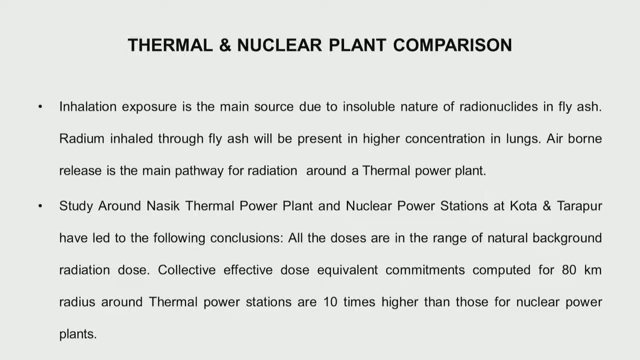 high concentration and they are inhaled, So inhalation is the main route. Okay, This is the way in which these radioactive products get into our system, and radium, of course, it has got an affinity for the lungs. It will get saluted in the lungs. 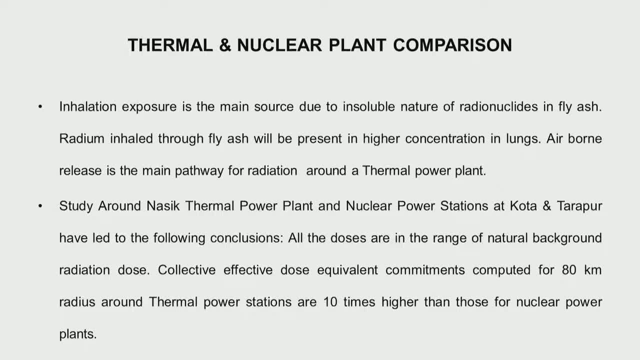 If it is iodine it will get in the thyroid, So this is the issue which needs to be kept in mind. So, overall, for a thermal power plant and nuclear power stations in India, research has been carried out And there are a lot of studies. 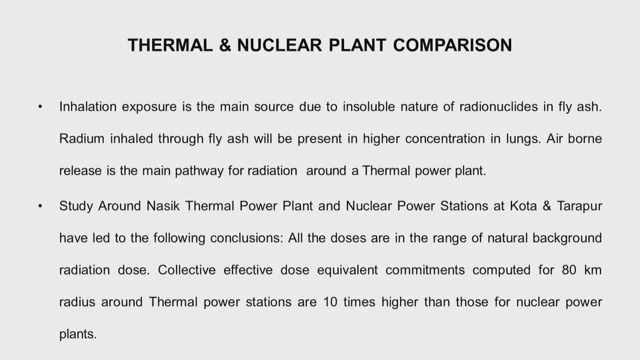 A lot of measurements have been taken based on the IAEA's guidelines And these studies, to summarize, have led to the following conclusions: that the doses which you are receiving, whether it is a natural nuclear power plant or a thermal power plant, around that, they are all around a natural background level, but the collective effective 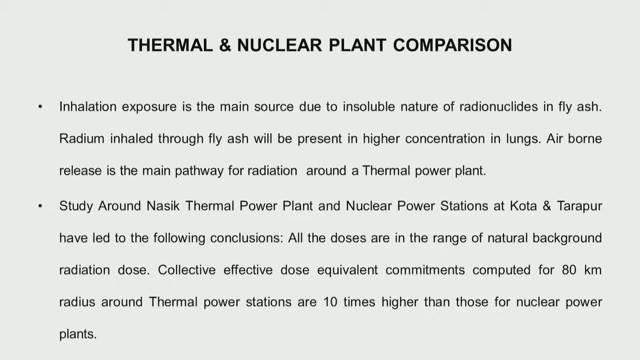 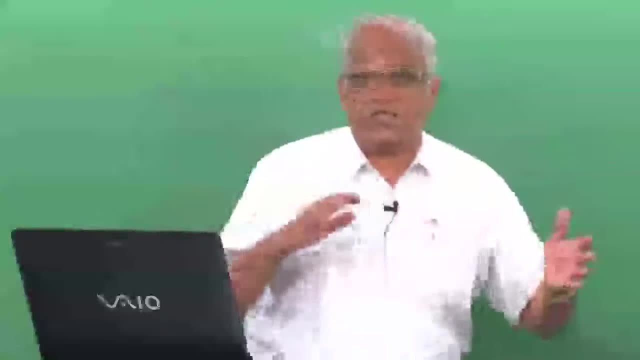 dose. If you compute for a 80 kilometer radius around a thermal power station, that is about 10 times than those of a nuclear power plant. It doesn't mean that, okay, thermal power plant is more hazardous than this thing. It is higher. 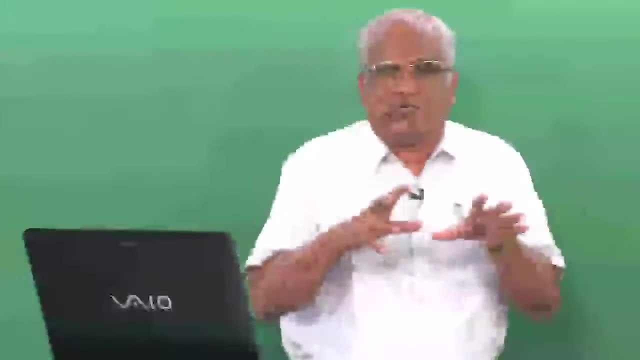 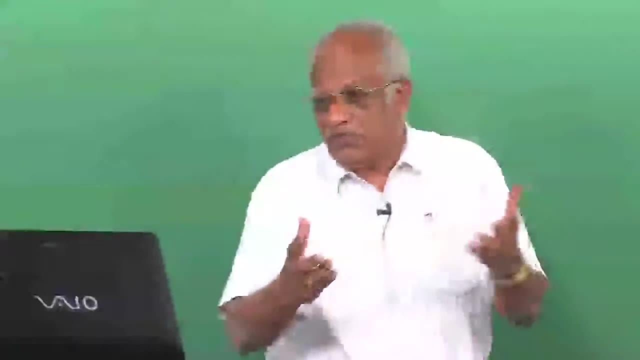 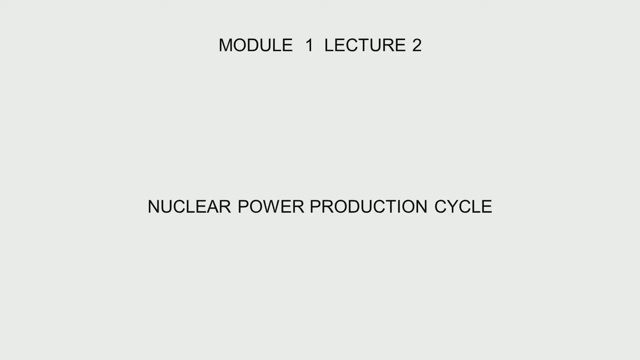 The only message which I would like to convey is: there is nothing to fear about living near a nuclear plant, that you are going to get radiation. So that's the main thing which I want to convey Now, having had an idea about the different uses of radiation. now let us go to the main. 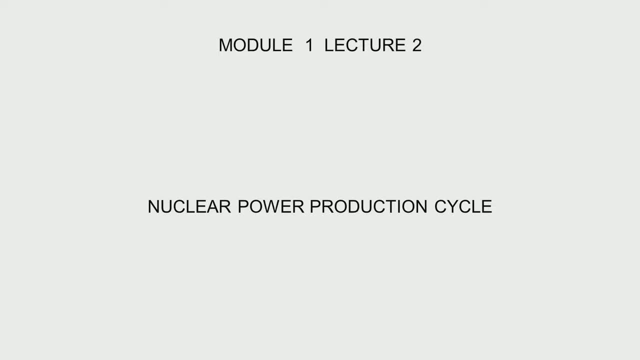 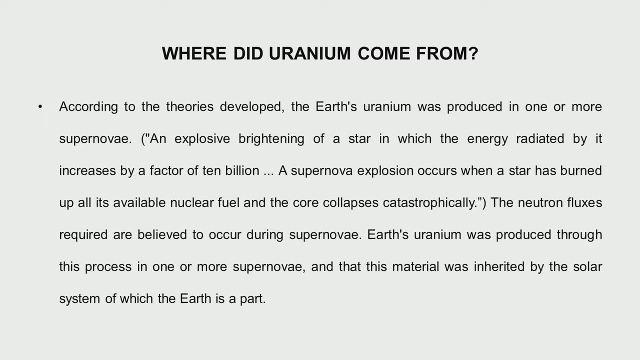 thing about which our topic is, on a nuclear power production. Now, to produce power, basically, we have one of the radioactive materials as uranium-235 that is available in nature. There is only one element, which can be fissioned, and that fission process produces heat and 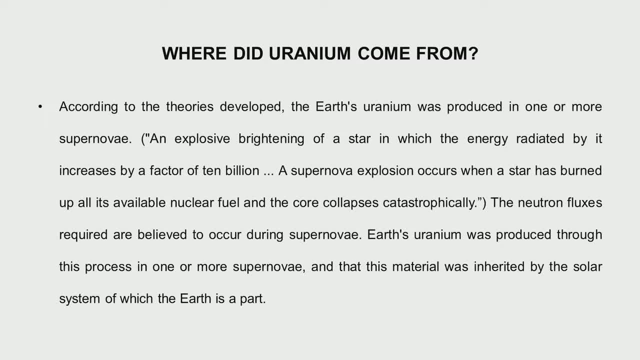 that heat is used to convert water into steam and run a turbine. Now let us have a look where this uranium has come from. As I said, it is naturally available, but perhaps the earth's uranium was produced in one or more supernova. 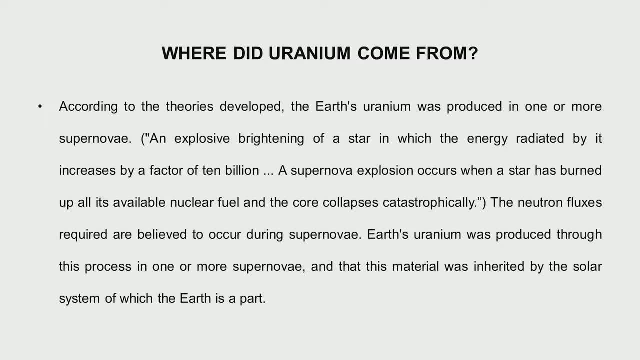 What is a supernova? It is an explosive brightening of a star in which the energy radiated increases by a factor of 10 billion. It is a huge release of energy. and when does a supernova occur? When a star has burned up all its available fuel. 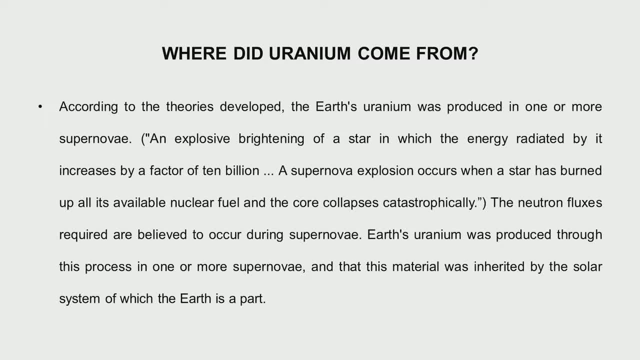 In fact, this earth itself was formed. It was formed by the big bang theory, in which the part of the sun exploded and formed the different planets. So earth's uranium was produced through one such process, and it is a part of our earth. It is not. 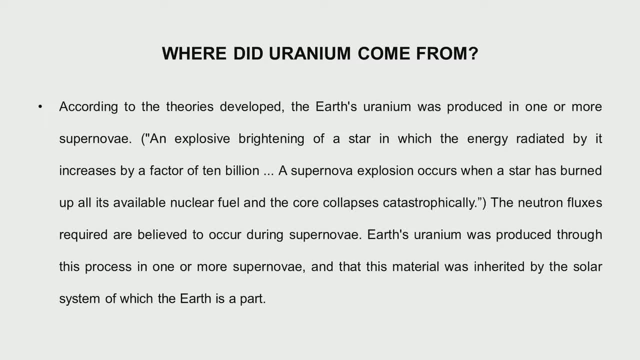 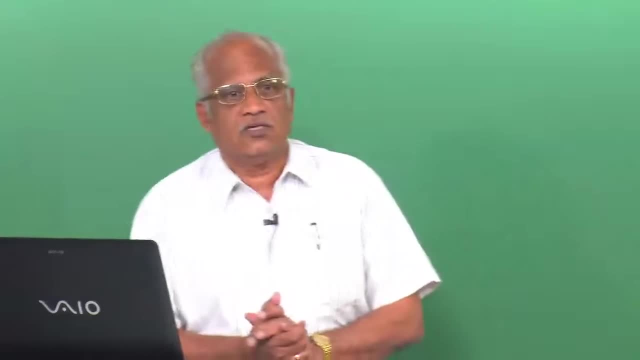 It is a whole solar system has. When I said the sun, there was a big bang. Sun is a fusion reactor, unlike fission. We will talk about fusion and fission later in our lecture. So this uranium is not manmade. Uranium has existed in a natural way in the earth. 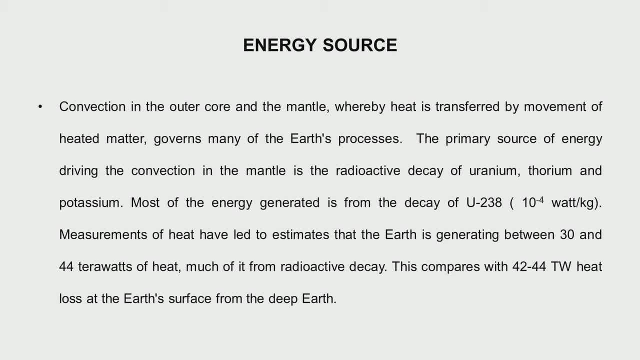 Now let us see what this uranium does. You know, we are living on the earth, whereas people are not able to live on planets beyond the earth: Mercury, Venus- Maybe it is very hot- Mars. We are thinking that some people may live. 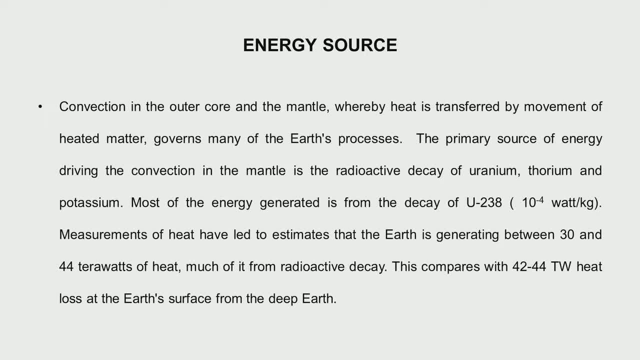 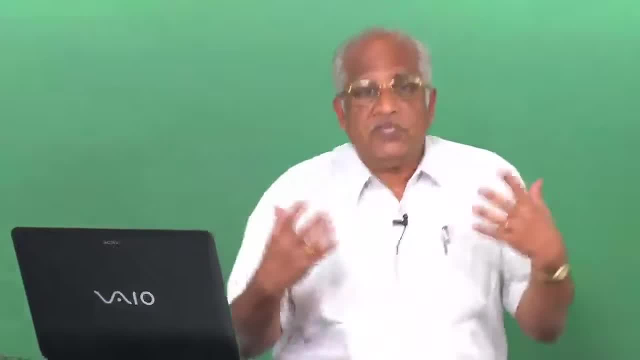 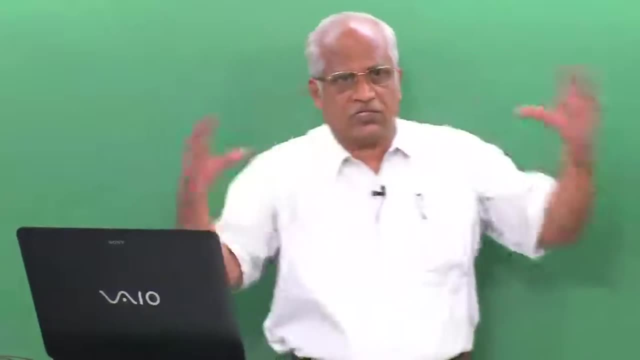 Jupiter, Saturn. Why? That means earth's temperature is very much suitable for us to live, So you require maintaining the temperature. If you look at the heat loss from the earth around which it dissipates, Is it? It is about 42 to 44 terawatt hours. 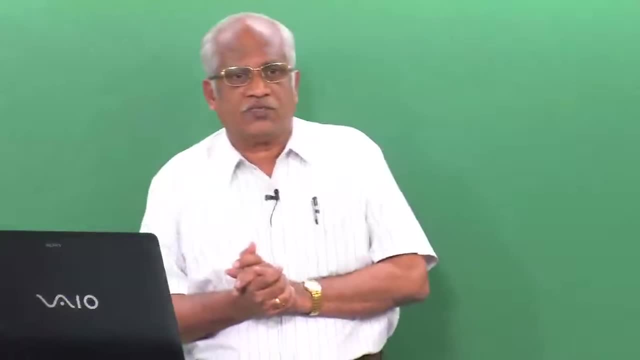 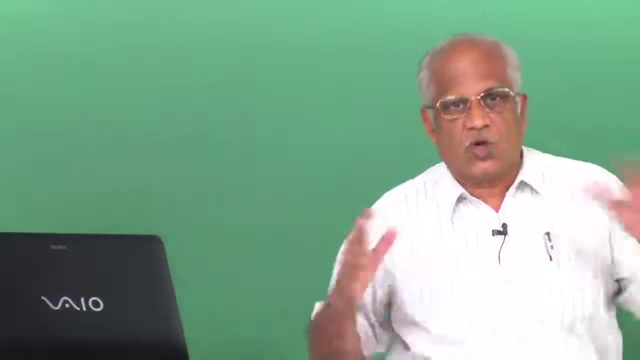 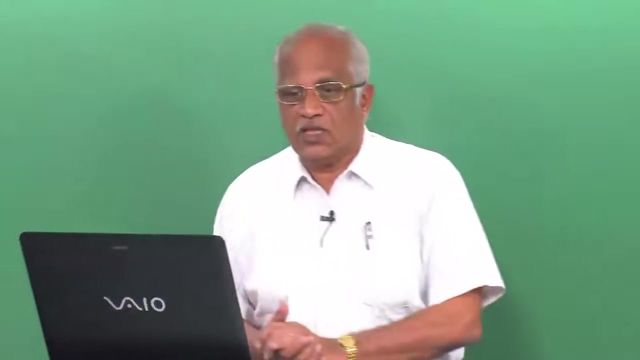 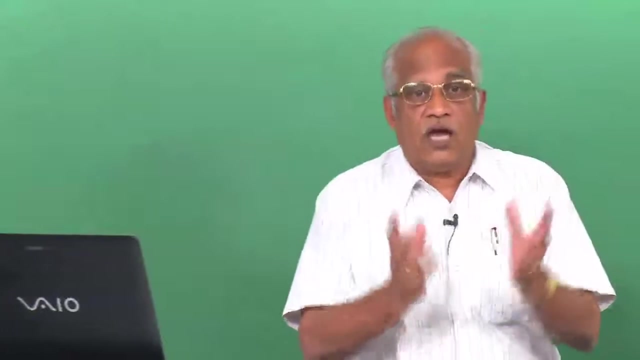 Terawatts of heat. It is happening from there, But this as the heat is lost. surely the planet should be cooling, but that is not happening. So what is happening? The heat is there because of the radioactive decay of the uranium, thorium and potassium. 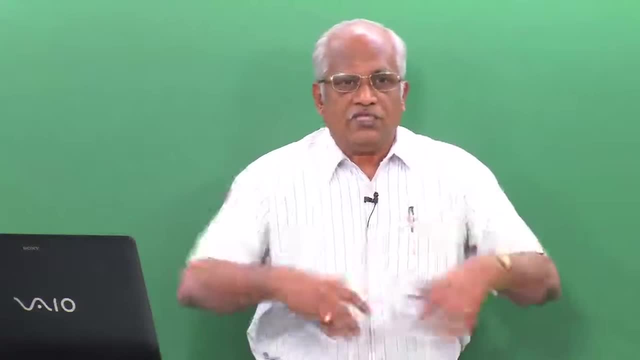 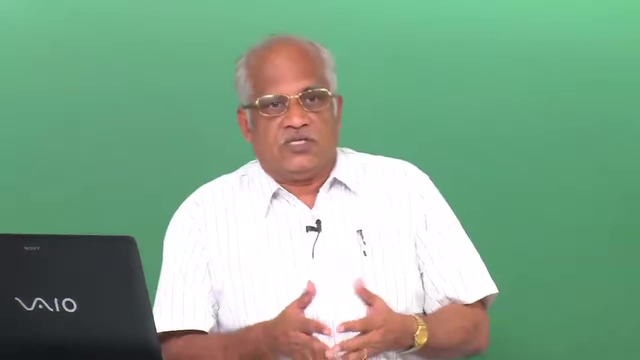 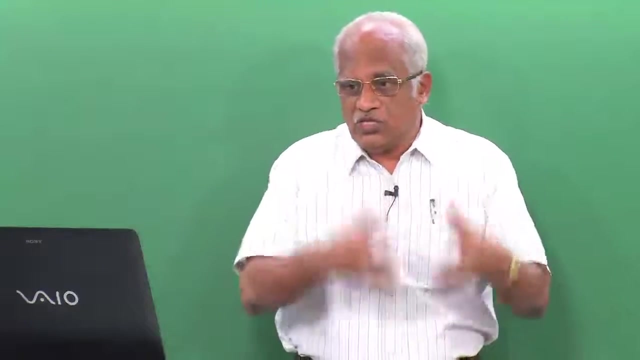 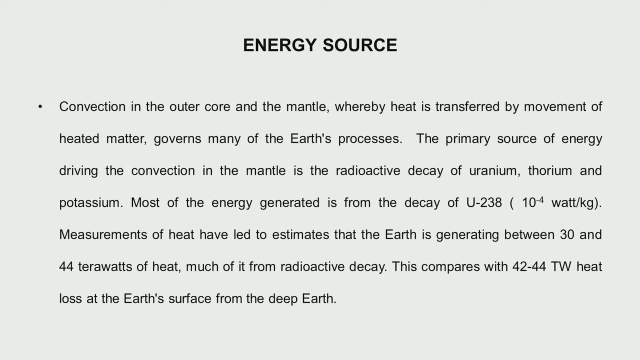 which is in the earth's mantle, And this energy is getting transferred to the surface of the earth through the our soil and other areas. So this way you can see, and the measurements of this heat which is coming out have shown that they are somewhere between 30 to 44 terawatts. 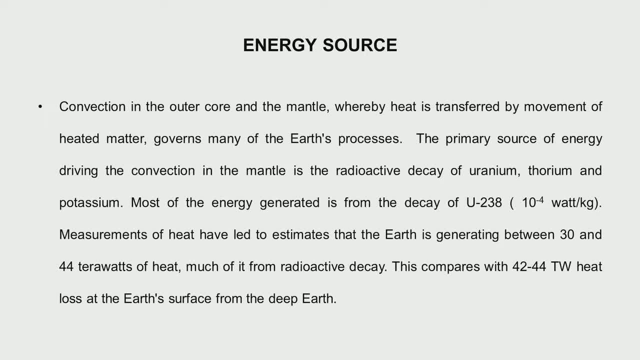 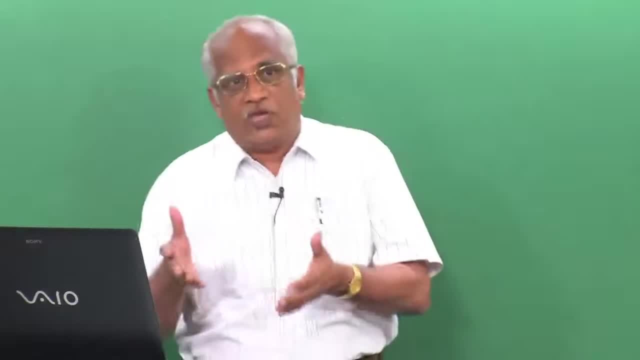 And if you just compare this number with the heat loss, You can get an idea. Maybe that is why we are able to survive on this earth, and the radioactive decay of uranium- The presence of uranium and its radioactive decay- is one of the reasons we are able to. 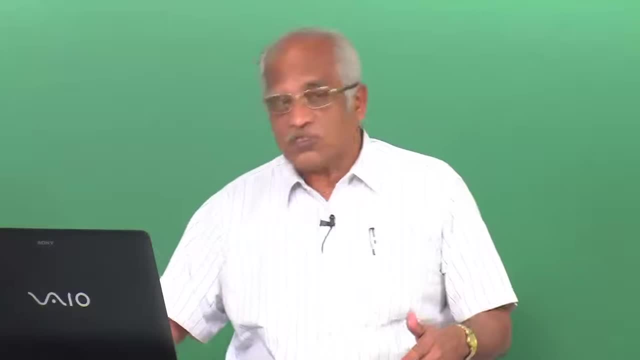 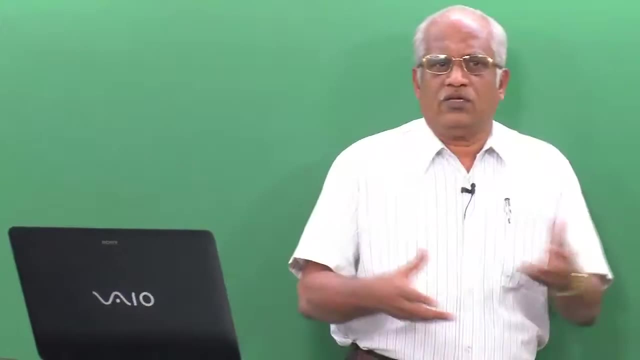 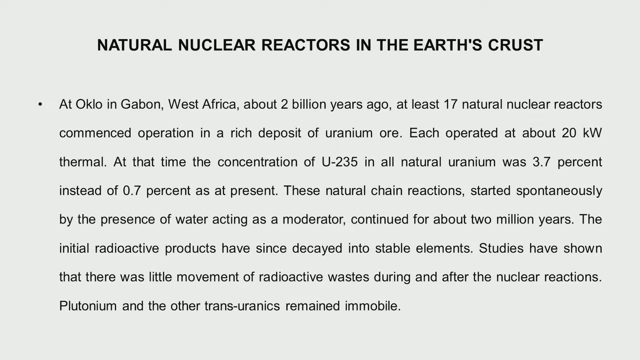 survive on this earth. Look surprising, but it is a fact. Then one might think: okay, The uranium is present there. Okay, Then this natural uranium in general contains 0.7% of uranium-235 and 99.3% is uranium-238.. 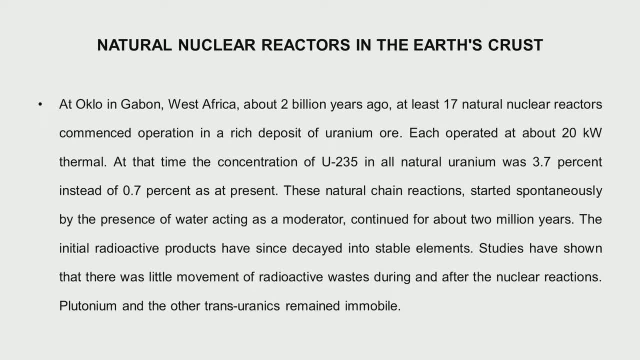 This uranium-235 is the only fissionable element which can be fissioned by a neutron. So apparently in West Africa there is a place called Oklo in Gabon. People did a survey of the natural uranium deposits which are there and they were surprised. 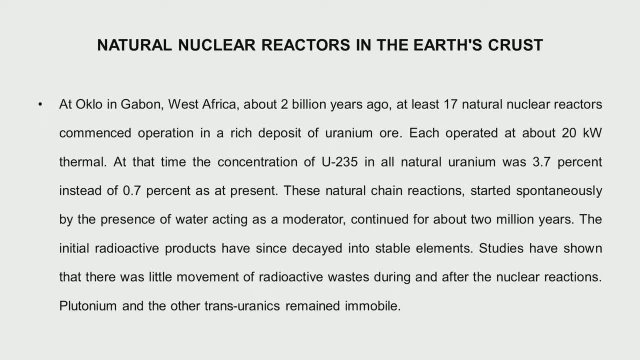 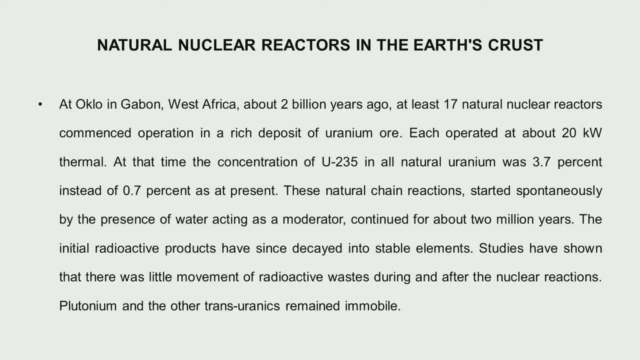 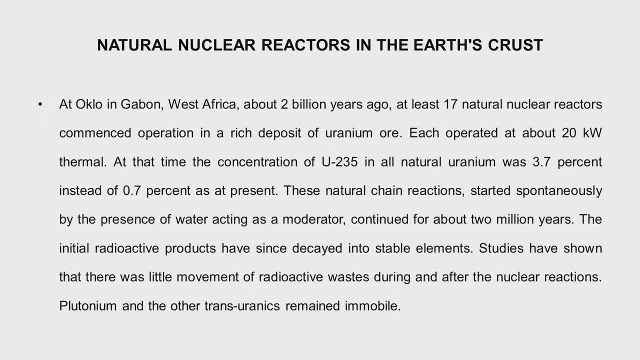 and these have been like a spontaneous reaction. Water has been there and the water has acted as a moderator and has been able to give Philip to the chain reaction, And this has continued for some million years, and many of the radioactive products that have decayed from these elements have been found in the in West Africa. 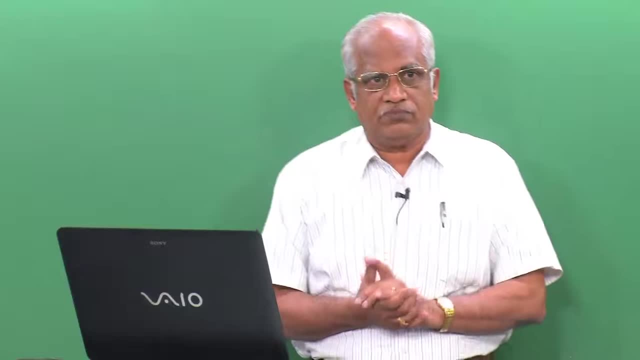 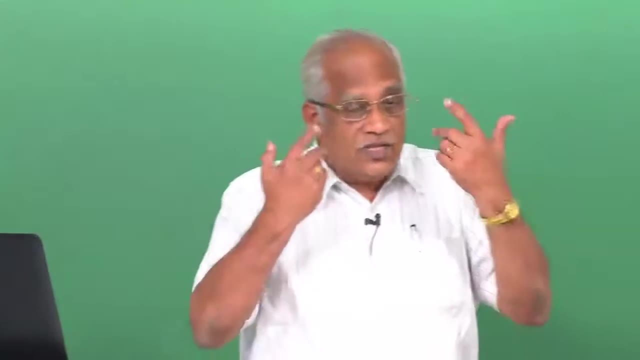 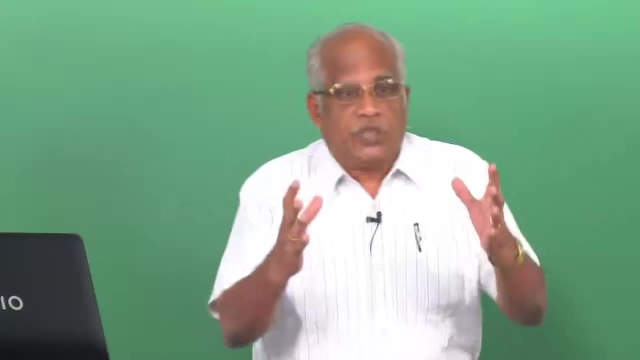 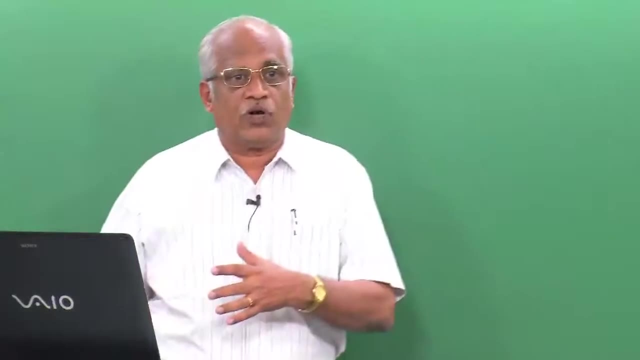 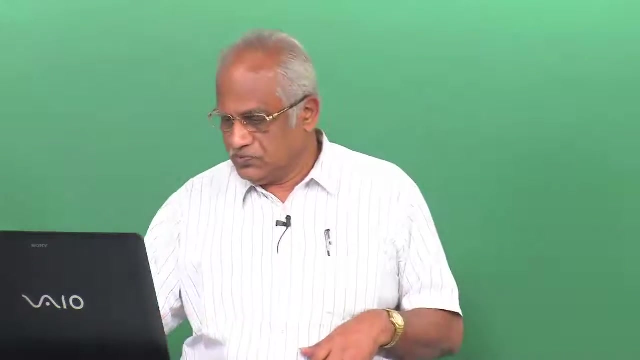 This was again one of the what you call inputs, And they found that even though you may put a radioactive material in the earth in a place, the earth itself acts like a filter. It doesn't allow the radioactive products to move about. So this concept has been very useful in waste management. 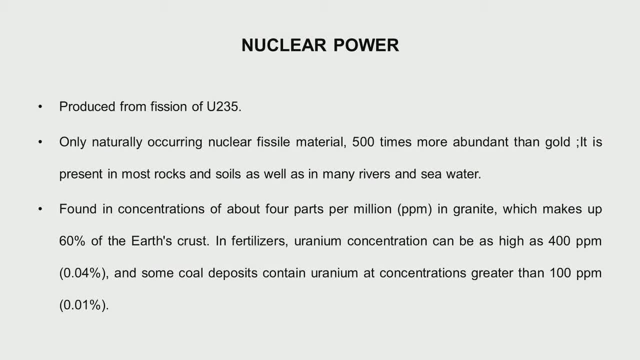 Coming to the nuclear power again, as I said, it is produced from the fission of uranium-235.. And if you ask how much of uranium is there, it is 500 times more abundant than gold and it is present in rocks, soils and everywhere, in water also. 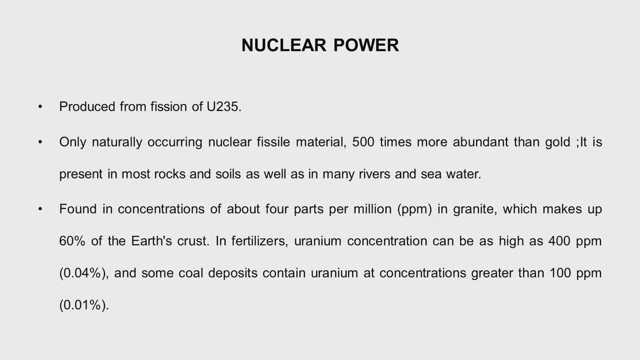 And in granite it is about four parts per million and you remember, granite makes up nearly 60% of the earth's crust. If you take fertilizers, uranium concentrations can be as high as 400 ppm And coal deposits, as I mentioned, they have concentrations greater than 100 ppm. 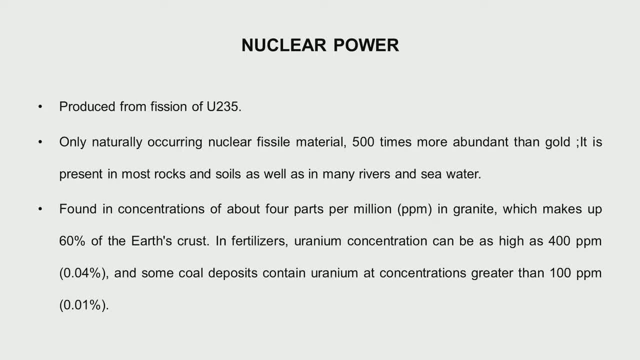 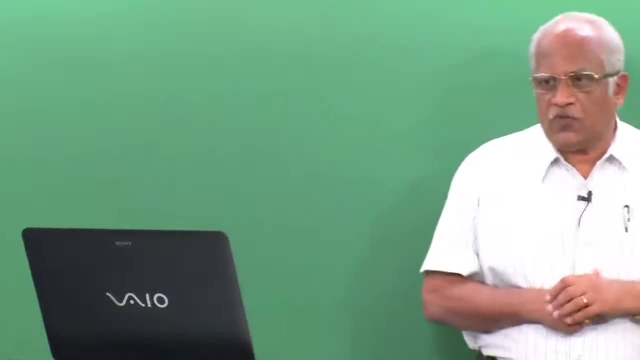 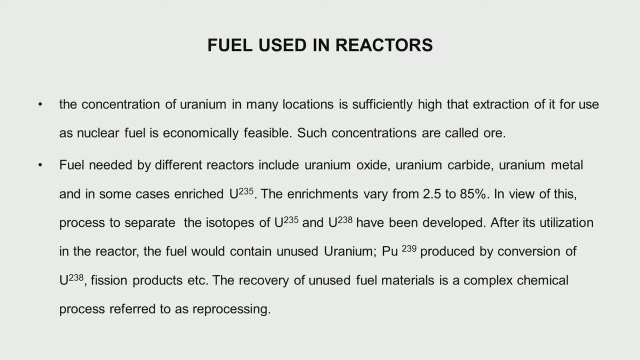 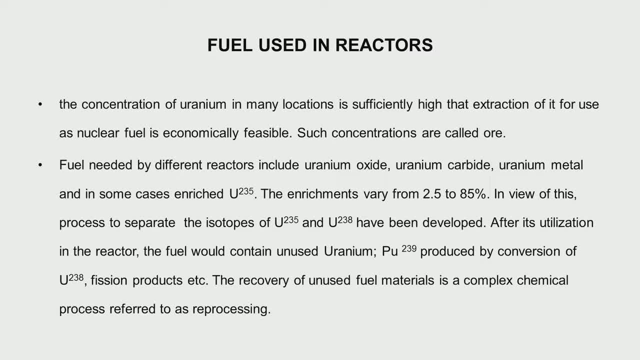 And this where the concentrations are high level. we call them as ore and then we start processing them to get the uranium. Now the enrichment of uranium varies in the. in the heavy water reactors We use natural uranium itself as a fuel, which contains about 0.7%. 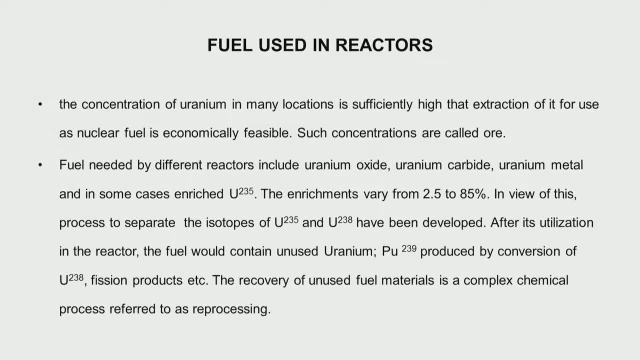 But most of the reactors in the world which are light water reactors. they use somewhere between 2.5 to 5% of uranium-235.. Okay- While the fast reactors use something like about 80% to 85%. So we have the need for development of process to increase the content of uranium-235 and 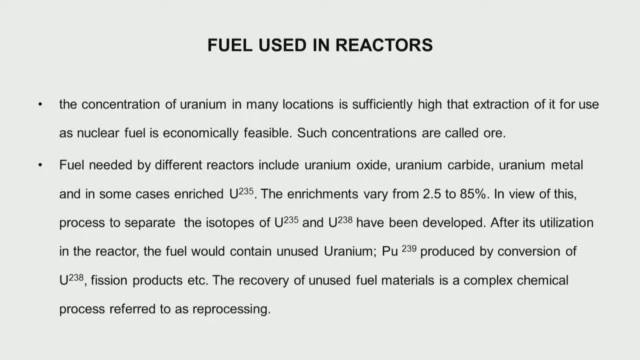 they have all been developed. Then after its utilization in the fuel- of course in the reactor it could be- the fuel could be uranium oxide, uranium carbide or uranium metal. Uranium metal was used in the initial reactors but due to its low melting point it was felt. 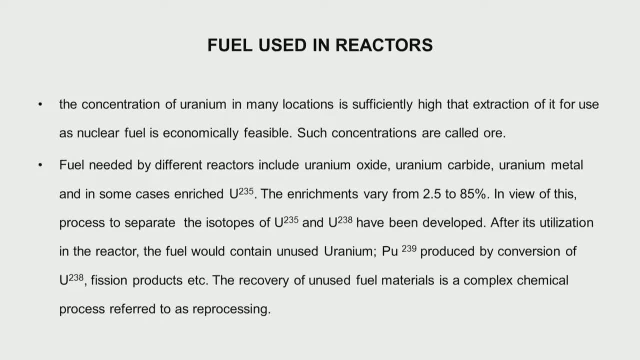 for to go to high temperatures, we should use a ceramic. So people went to uranium oxide, which has been very widely used. Uranium carbide also has been used. Now, once the fuel has been utilized in the reactor, Then some unused uranium. 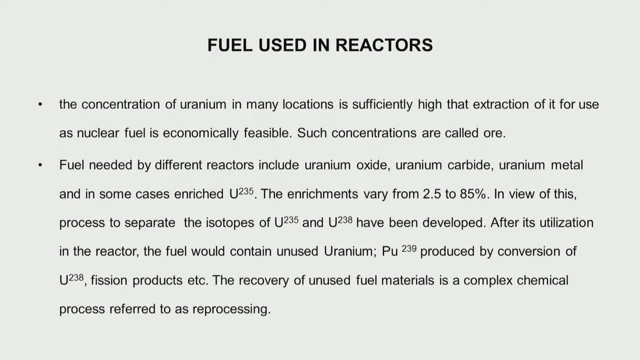 Surely not all the uranium would have been utilized. and then plutonium-239, which is produced by conversion of the uranium-238 and some fission products. So this uranium-238, which is 99.3%, gets converted to plutonium 239. and this plutonium-239, luckily, 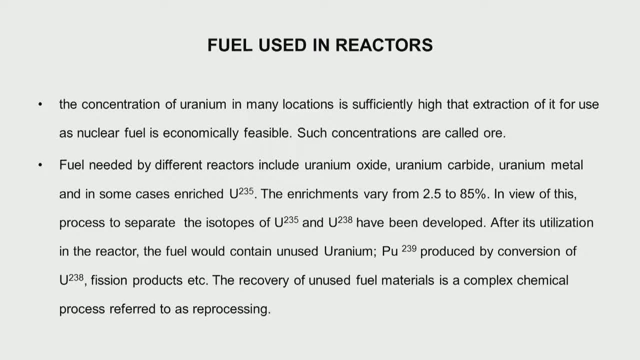 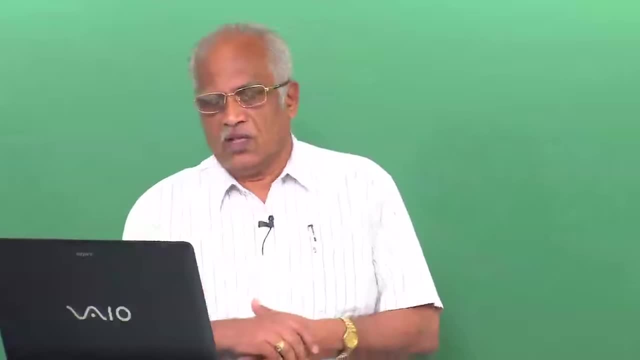 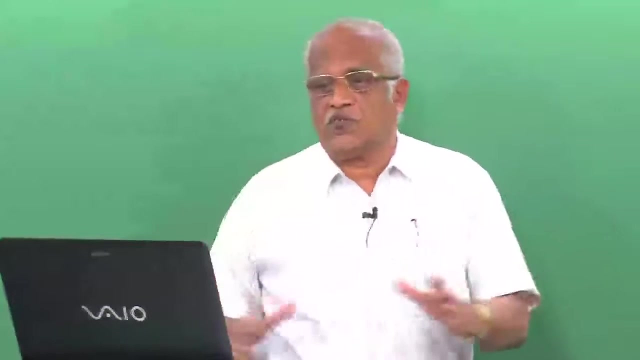 is again fissionable, So this is a man-made fissile material. In the recovering this, plutonium-239 and unused uranium is what we call as reprocessing. This is a word very frequently used: reprocessing. So now you can get an idea about the full cycle through which the fuel goes. 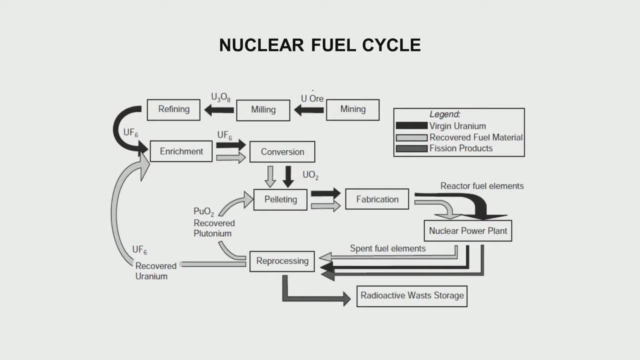 You start with the mining, get the mine, get the uranium ore. Then you go through a process of crushing and refining. Then you have a stage of enrichment. Then, in case you need to have to more than 0.7%, you have to enrich it. 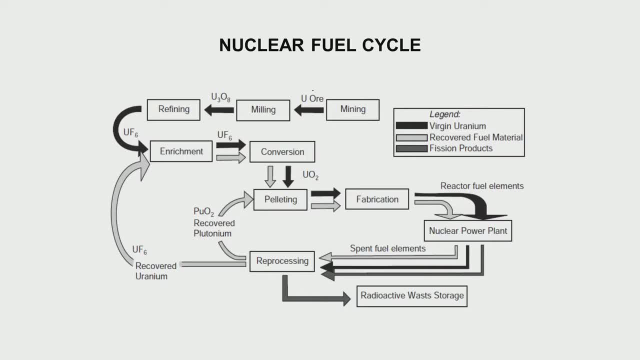 Then you have to convert it into the form of oxide. Then these fuel which are in the powder form, they have to be put into pellets, and then pelletizing is one, and then made into fuel elements and used in the nuclear power plant. And from the nuclear power plant it goes to the reprocessing where the plutonium-239 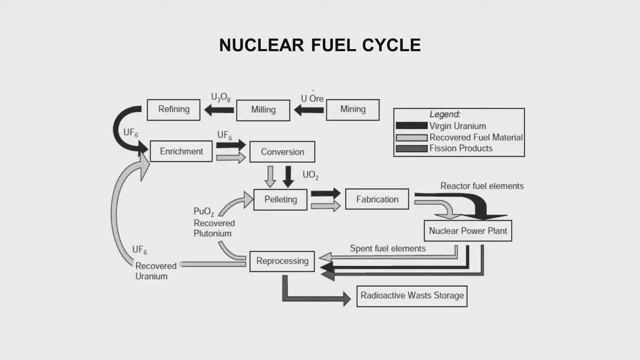 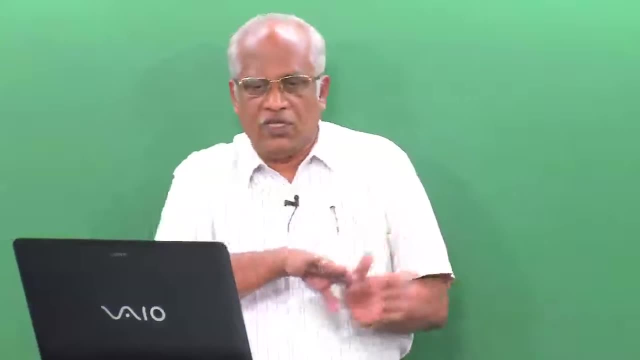 and unused uranium are extracted and they are sent back for reconversion And again fabrication to be used in the reactor. And whatever is not, the fission products and all which are after the reprocessing. they are to be called as a radiation waste and stored properly. 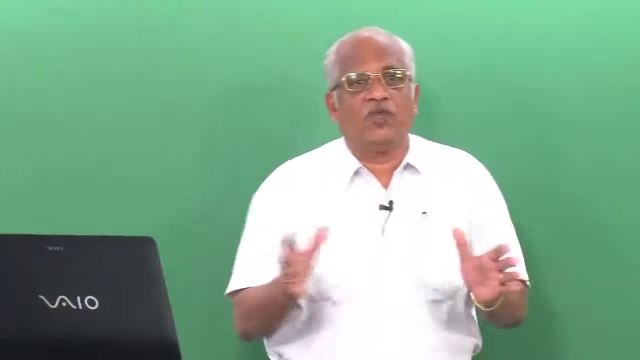 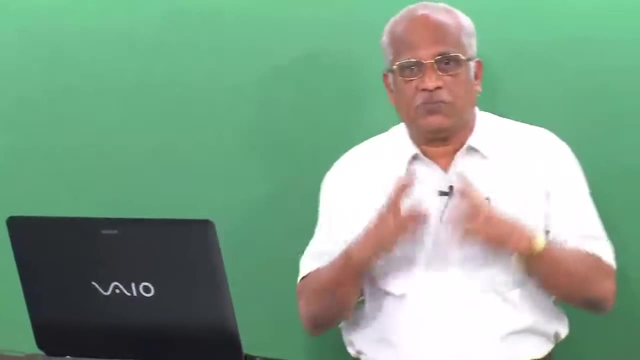 So this is the nuclear fuel cycle in a very brief manner. To get an idea of the quantities involved- because that is very much important- you must know what your material amount of material is. So this is the nuclear fuel cycle. This is the material you are dealing with. 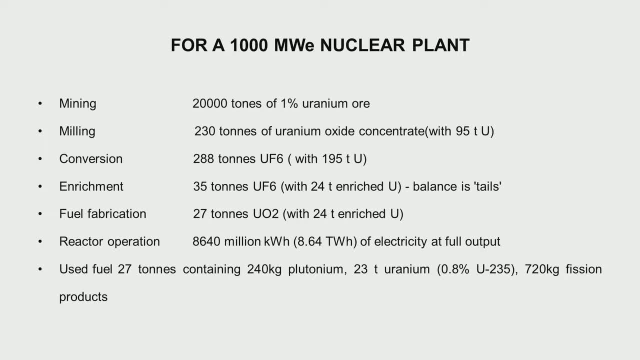 Let us take a 1,000 megawatt electrical nuclear power plant. Now for that you have to suppose we consider a ore containing about 1% uranium. You require about 20,000 tons of uranium ore you have to mine and 230 tons of uranium oxide. 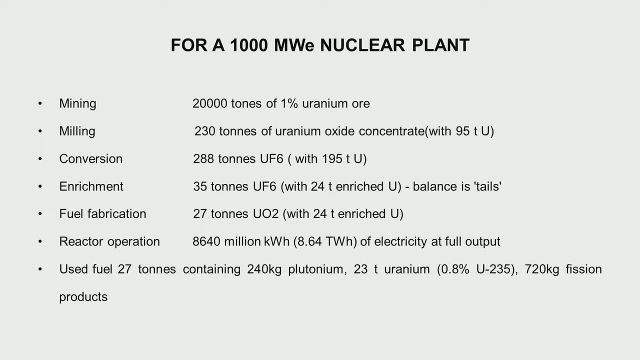 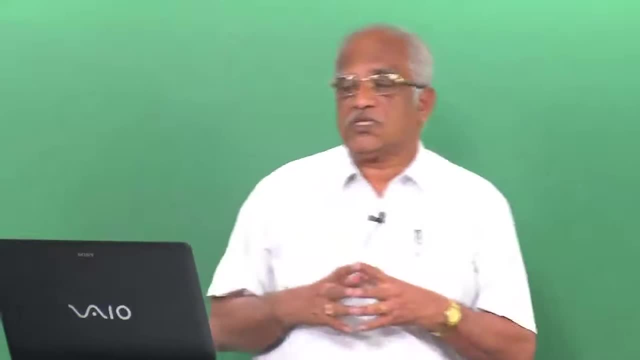 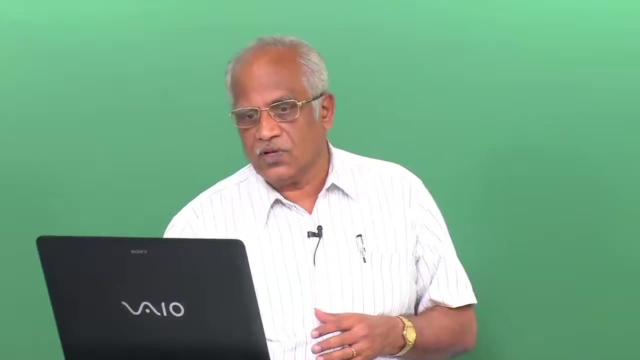 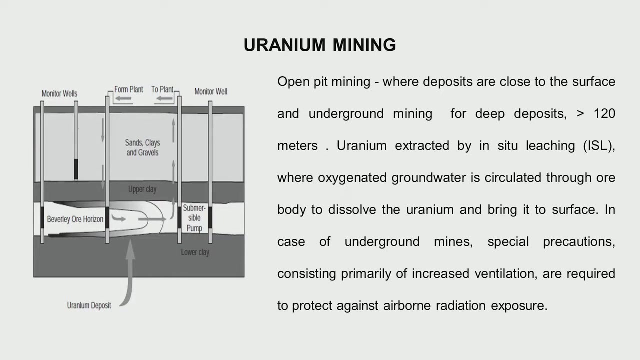 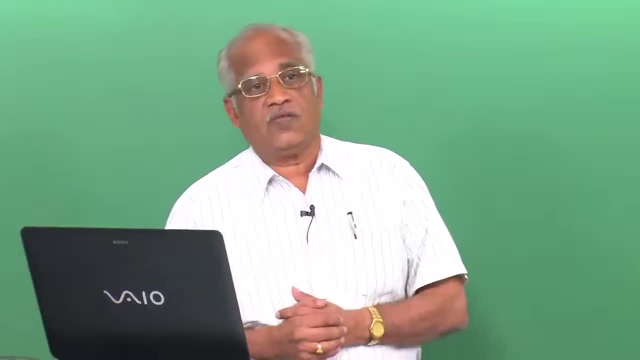 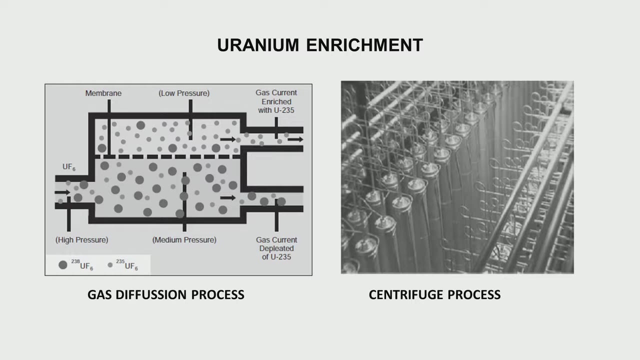 Then we have the enrichment process. The enrichment consists of two methods. One is the gas diffusion process and the other is a centrifuge process. Now, in the case of gas diffusion process, we use basically principle of diffusion, and it has been quite effective. 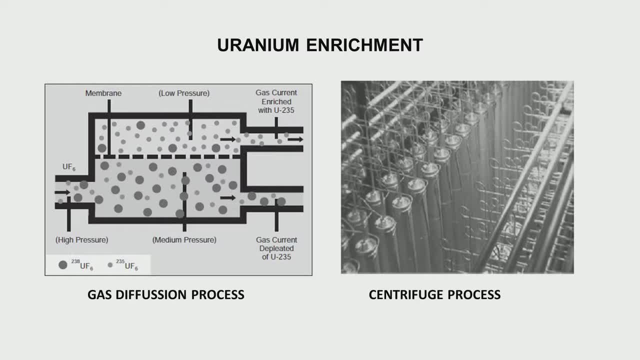 The other process is basically using the centrifugal force- what we call as a centrifuge- running at about 70,000 rpm, wherein the uranium-235 and 238 get separated and then you are able to take out the enriched uranium. But the centrifuge process is quite power intensive. 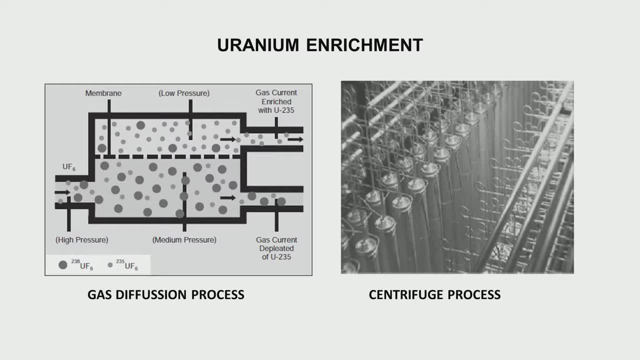 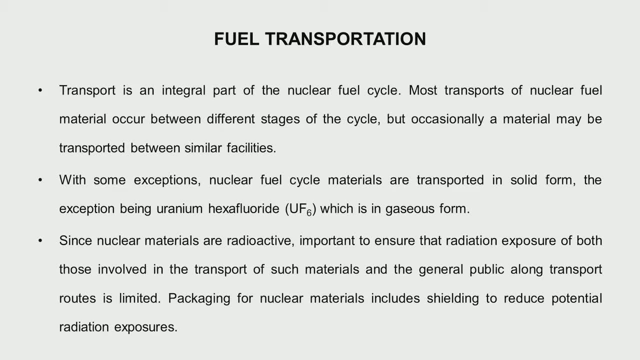 So that is the reason why many countries have not been able to go ahead with this Already. they are in need of power. Okay, Then this fuel has to be transported. When I mentioned to you about the carbon dioxide emissions from the new in case of nuclear, 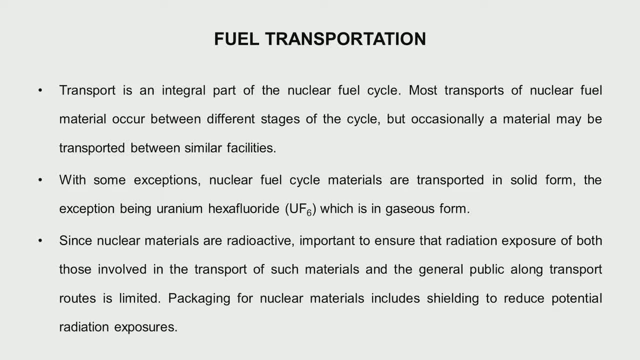 power plants. whenever we manufacture and transport a component, it has to come on a diesel vehicle which is going to have carbon dioxide emission. So transport is very important stage in which the nuclear fuel will move between different parts of the cycle. So you have to be very careful. 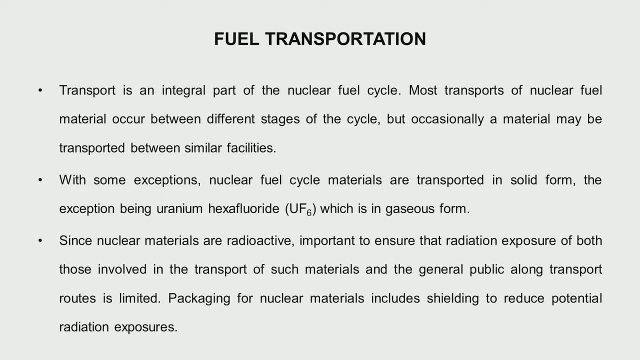 So that during the moment this radiation exposure should not affect the people who are involved. It should not affect the public. So we have to see that they are packed properly, shielded properly. We use the word shield radiation, shielding materials. we use so that effect of the radiation 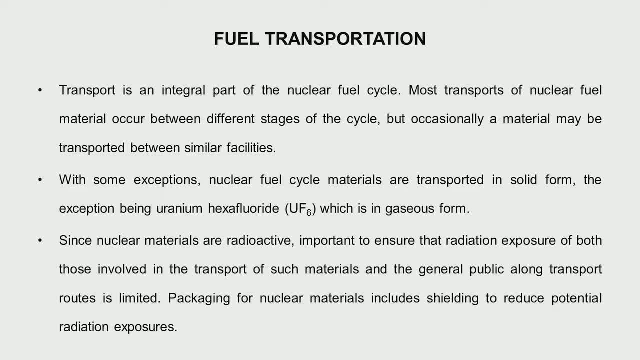 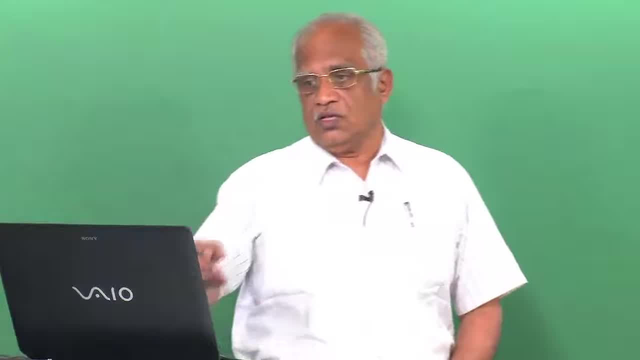 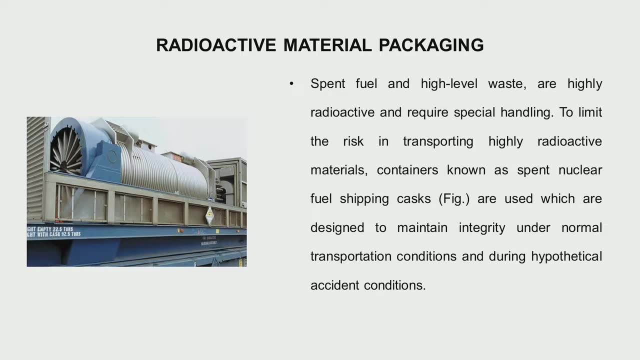 is not felt outside. So these are the safety measures which need to be involved in the transportation. Okay, Just to give you an idea how a cask containing radioactive material looks like, this is: see the cask which is mounted on the train. 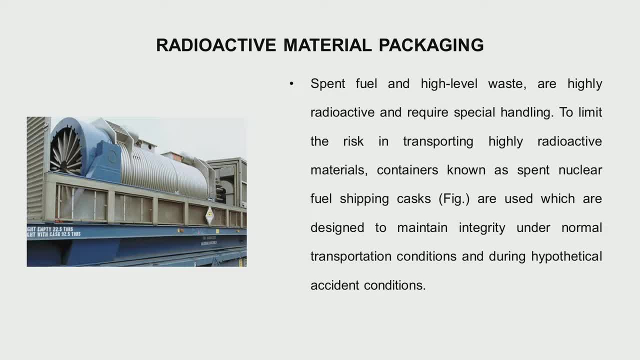 You see, it is a goods train. It is mounted and this contains waste or raw materials. also, This particular one contains waste, nuclear waste, which is also radioactive, and this design is done in such a way that these casks, even if they fall down, they won't break. 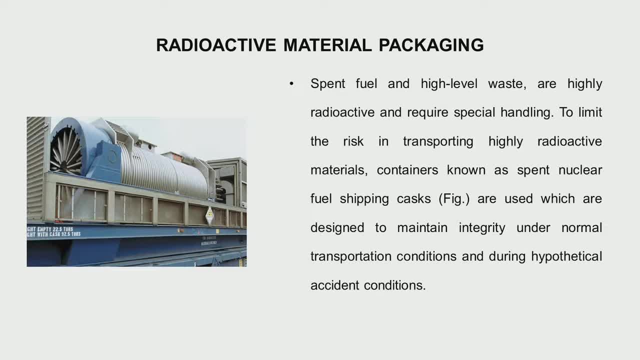 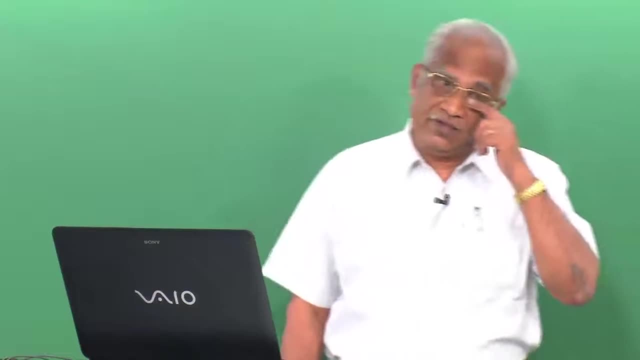 You will be surprised. in the United Kingdom in the 90s, there was a one person raised a question. Suppose this train carrying this radioactive material or radioactive waste meets with an accident. what will happen? Believe it, they took a train with one or two containers. 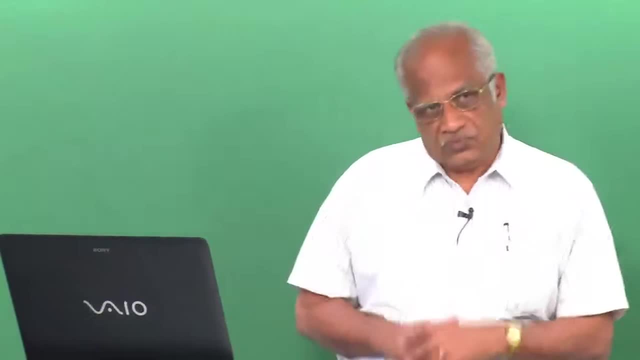 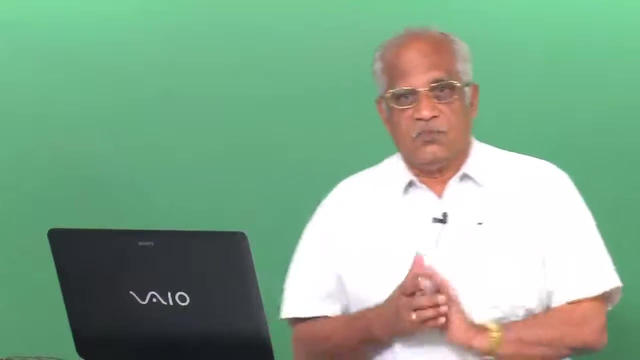 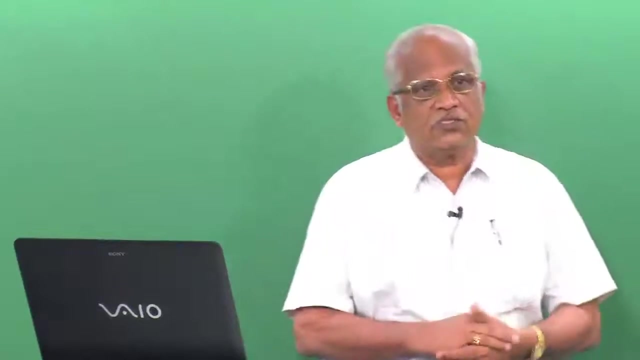 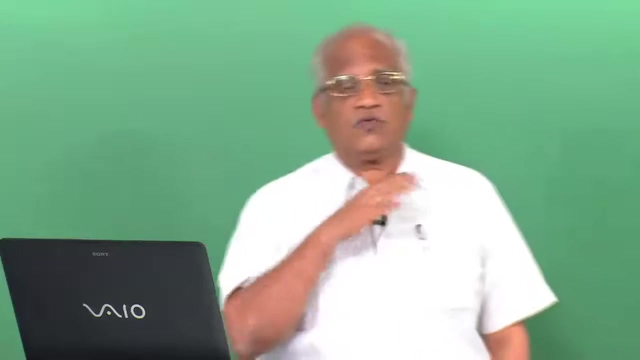 Containers and containing the radioactive material, and the train really was made to have an accident and the cask fell down and nothing happened. So one thing is sure: the methodologies which we are adopting for radioactive material are good and we have to need to. the need is that safety at every level. of this we should be. 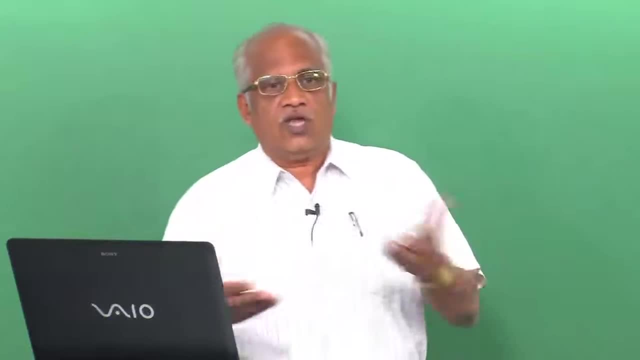 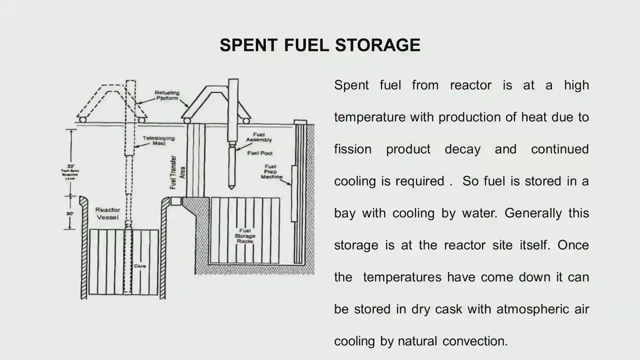 safe, So that radioactive releases or the radioactive contamination to the public and workers is minimal. Then the spent fuel. Let us take the spent fuel. The fuel has been used. Now you have to take it out, But it is at a high temperature. 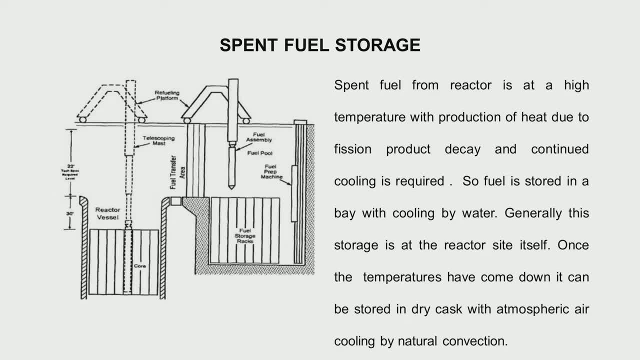 It is not in a temperature in which you can hand it immediately, So it needs to be cooled. It has to be put in a you know with proper cooling. Then only If you don't cool it, Then that fuel itself can melt. 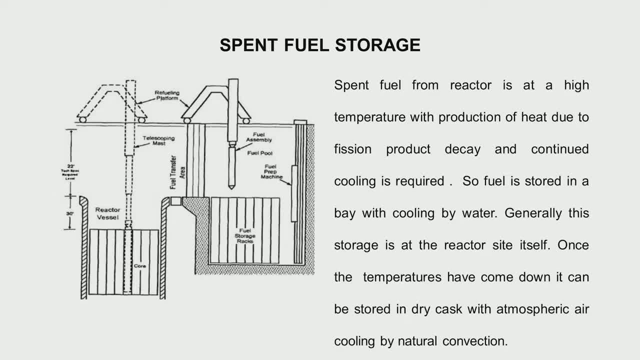 So normally we have a spent fuel bay in which we put the fuel, and you can see a simple system wherein, from the reactor core, the fuel is handled and then put to the spent fuel bay. One more thing is important: that the geometry of the fuel bay and water should be such that 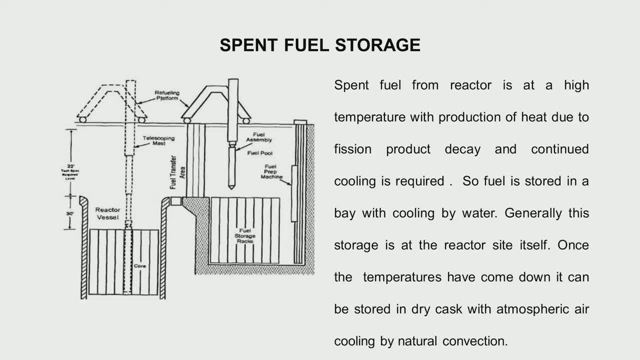 it should not become critical. Okay, We will see about this later. So this storage has to be kept for some time until the temperature comes down. Then, in a dry cask, you can transfer it to the reprocessing, and during that time, when you transfer it, even natural convection of air could be sufficient to cool the cask. 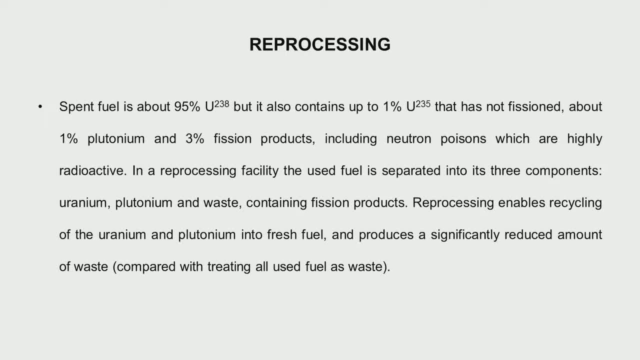 Then, as I mentioned, reprocessing. Okay, So you can see that, And the spent fuel is about 95% uranium-238, because all the uranium-238 doesn't get converted into plutonium, Only part of it gets converted. So also it contains about 1% of uranium-235 which has not fission. 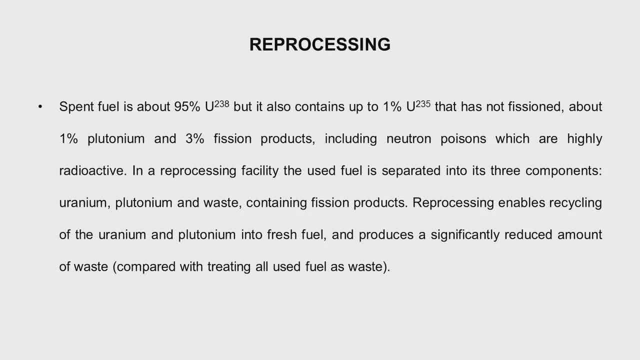 1% plutonium and about 3% fission products. Besides you have neutron poisons like xenon etc. which may be there and they are highly radioactive. So in the reprocessing you separate the components. Basically we are looking for taking out uranium, plutonium and the waste containing the fission. 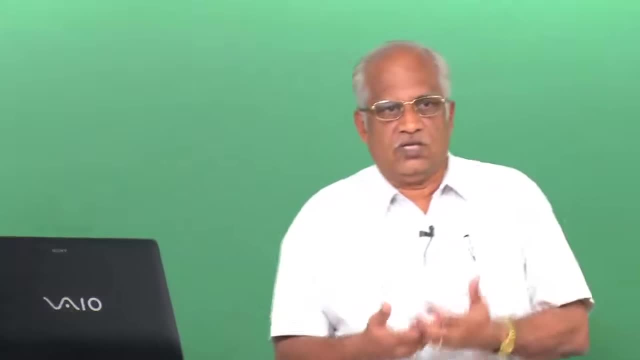 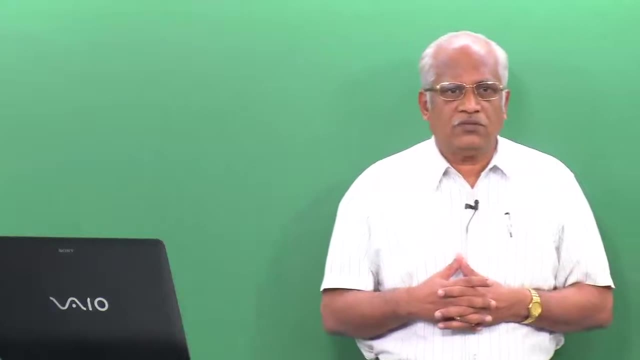 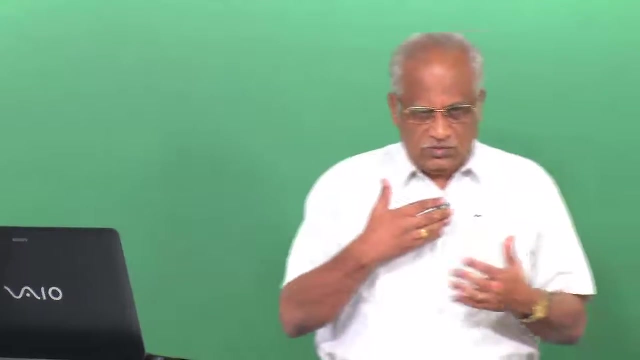 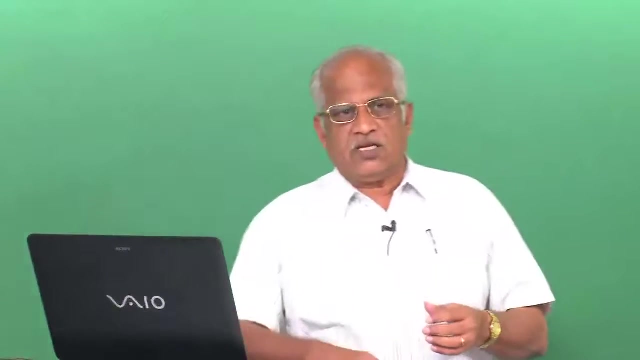 products and, based on the reprocessing output, we can use the uranium and plutonium into fresh fuel and so that it is effectively, we are reducing the waste. Now You might wonder: Okay, But in the media there has been always thing that reprocessing should not be there. 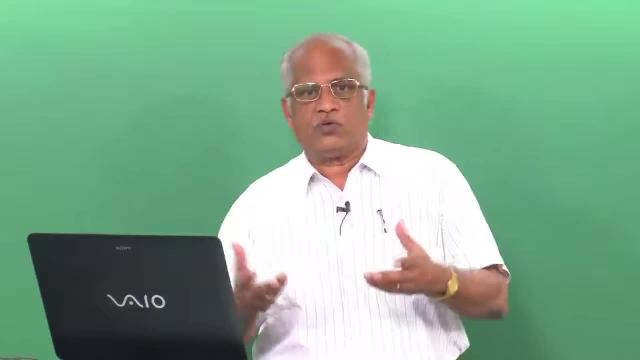 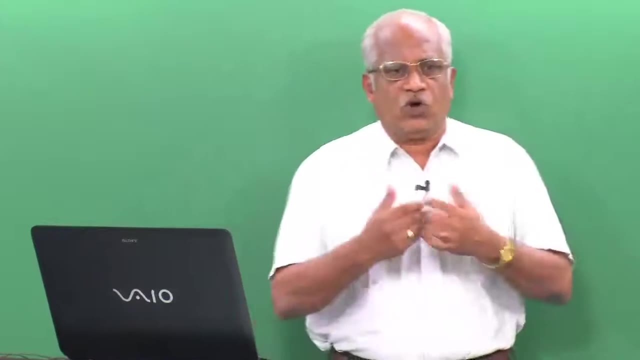 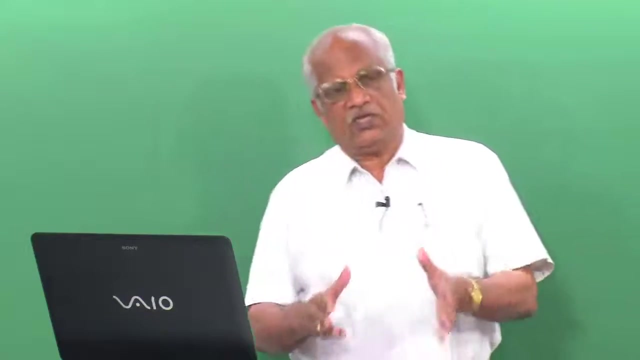 Reprocessing. we can lead to proliferation. we can- people can- take the plutonium. Now USA has adopted this attitude that whatever is coming out of the reactor, it is not used again, it is just kept as a waste. but in this process the waste activity is high because 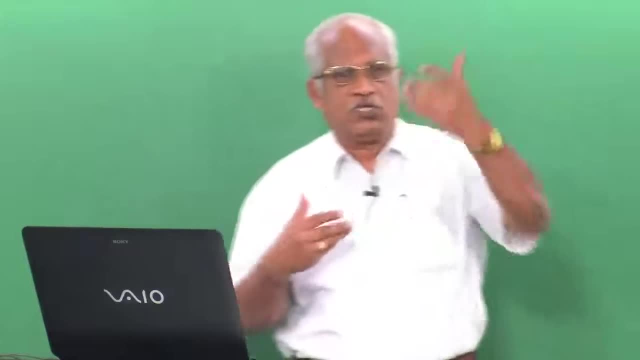 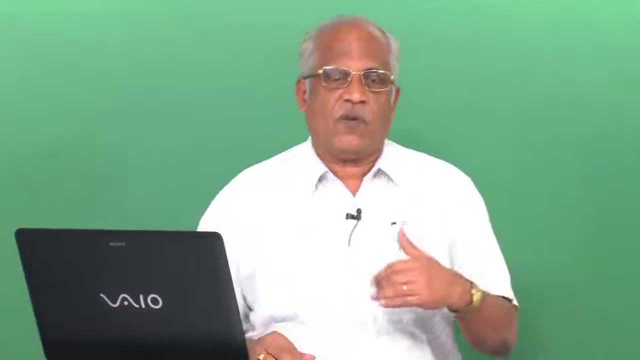 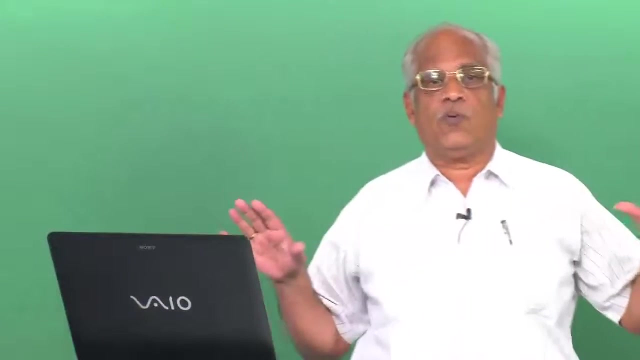 of the presence of uranium and plutonium. if you can separate it and then use it in another reactor, you are effectively utilizing the resources. In fact, this type of approach without reprocessing is called generally as open cycle, open fuel cycle, whereas what I was talking about, the nuclear fuel cycle which is used back it is 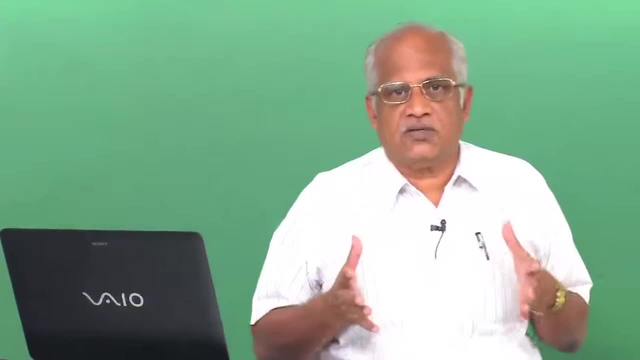 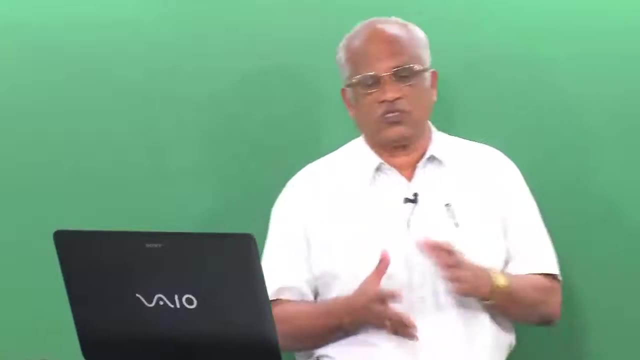 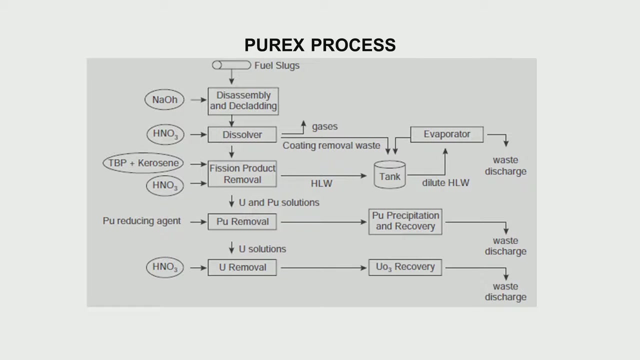 called a closed fuel cycle, and India per se Has gone in for a closed fuel cycle, But because we want to effectively utilize all our natural resources of uranium, There is a process, which is a well-known Purex process, which is used in reprocessing and 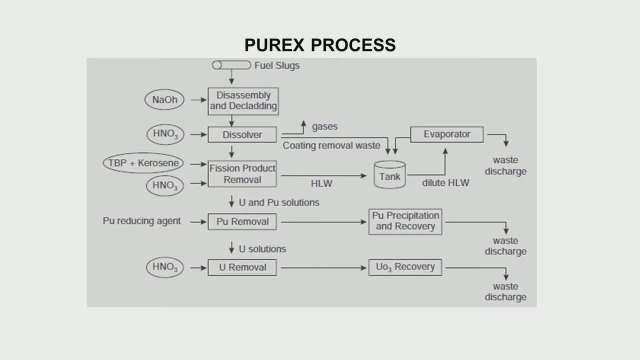 just to get an idea, what is the components of the Purex process? you can have a look at this figure. It is a schematic figure in which it involves the disassembly of the fuel, the decladding. remove the cladding material of the fuel, then dissolve it using nitric acid. 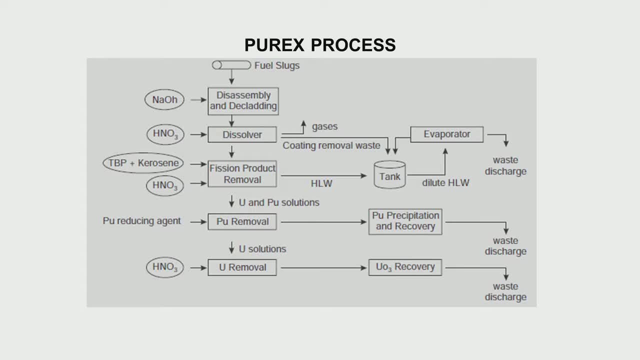 Then to extract the fission products they use TBP plus kerosene. it is tributyl phosphate and kerosene along with nitric acid. Then whatever is removed then goes further. You get uranium and plutonium come in solution form. 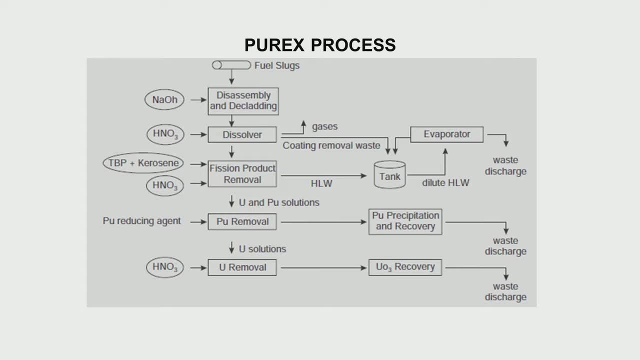 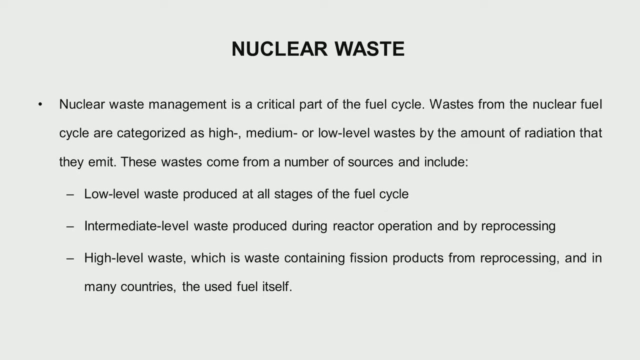 Then you remove the plutonium and uranium separately. Whatever is the rest in the second stage after the TBP, what is does not get dissolved is sent as high-level waste and, of course, the rest of the process is, as shown, okay, Now the waste which is coming out from the reprocessing plant. what we do? it is a very 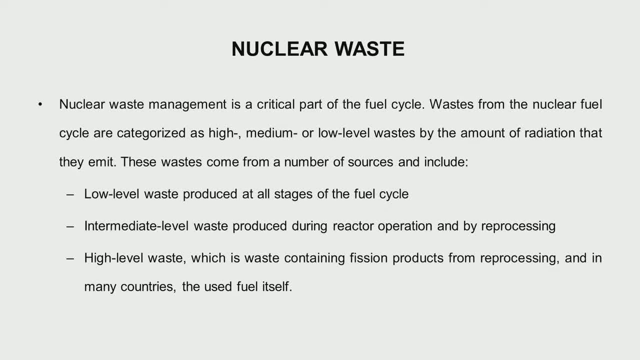 important part of the fuel cycle. We normally try to categorize them as high-level, medium-level or low-level, based on the amount of radiation. Now, low-level waste are practically produced at all stages, like right from mining, then your fuel fabrication, everywhere they are all produced. 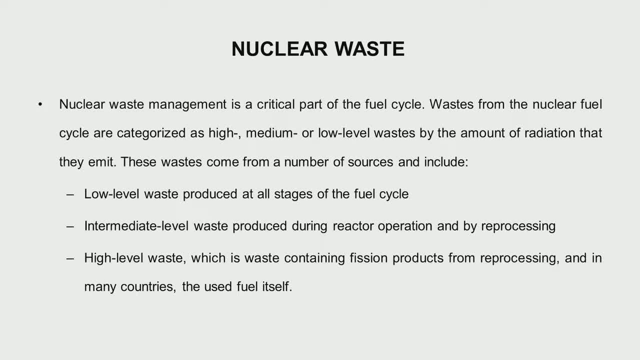 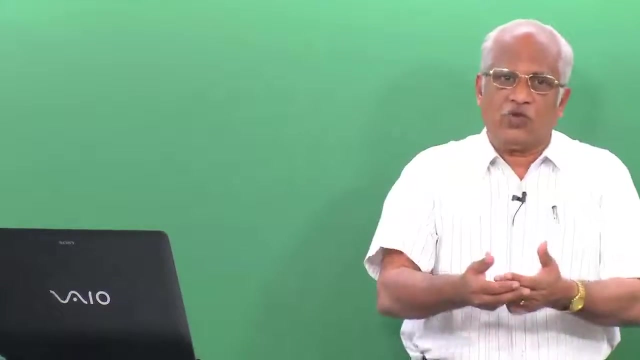 Then intermediate-level waste are produced during reactor operation or by reprocessing, Okay, And the final high-level waste is basically from the fission products which are taken out in the reprocessing plant, and that is which is called as the high-level waste. Now, this is high-level waste, is the one which we are saying that we can use back in the 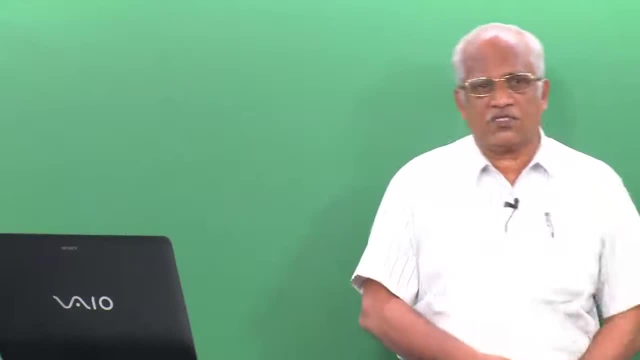 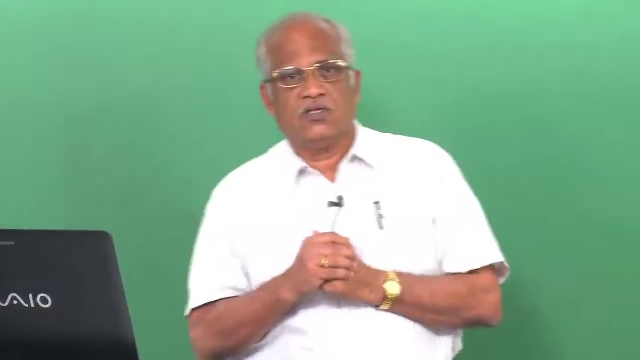 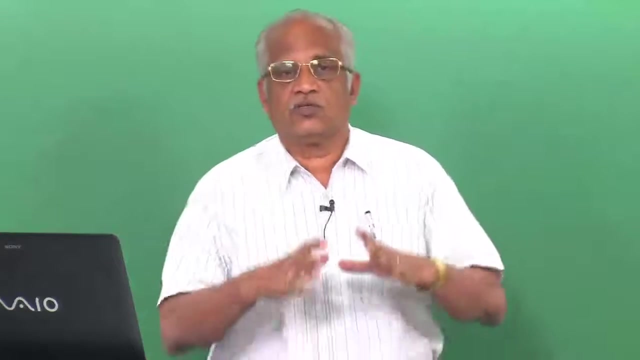 reactor so that we do not have any high-level waste To get and fill of this high-level waste. how much would be the quantity of high-level waste? Very simple example I can give you. Suppose one person's requirement of electricity throughout his life was to be produced only 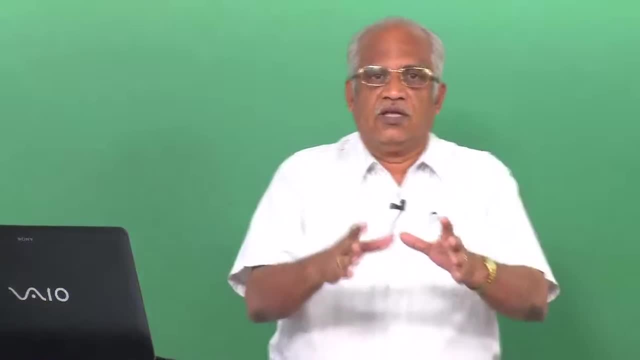 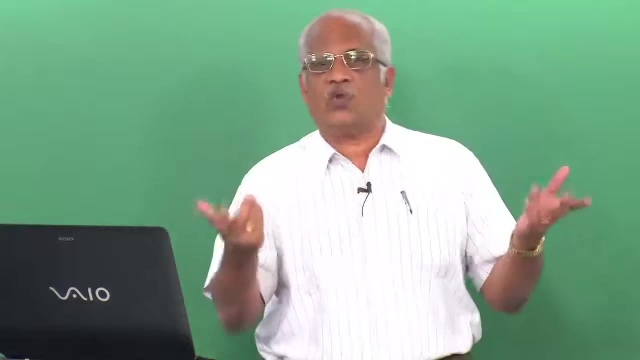 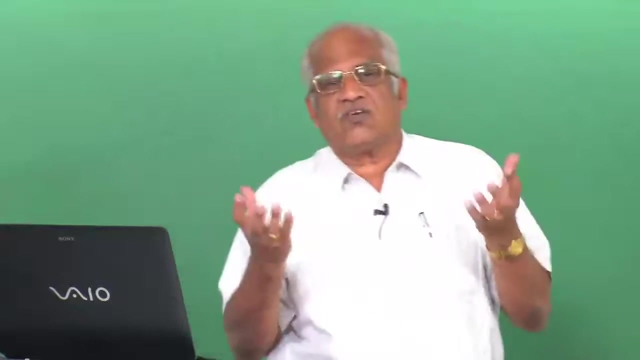 through nuclear power, then the high-level waste will be equal to one fist. That is all, And that itself, if you again put into the reactor, there is no high-level waste. So there is a fear that this high-waste management is very difficult and things it is not the 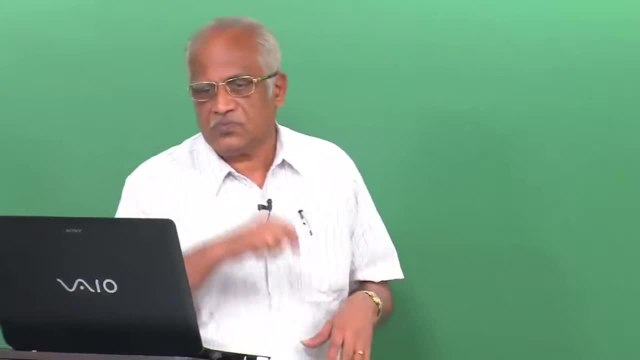 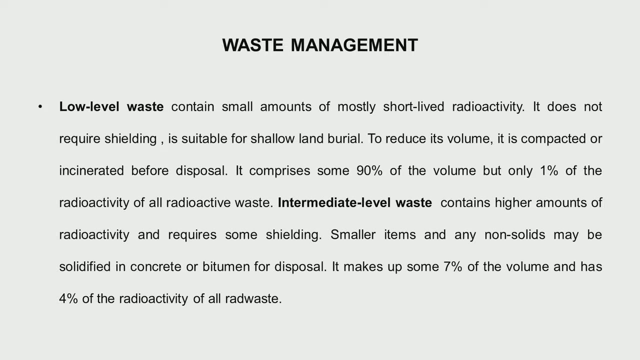 quantity, It is less. Now how do you manage this waste? Low-level wastes contain radioactivity, but this radioactivity is having a very short life, So it is not very much. It does not require a shielding and it can be just buried under the earth. but before 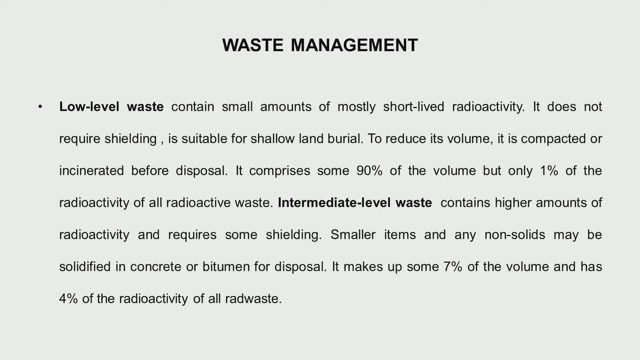 burying up. we just try to compact it So that And we also incinerate so that those material which are can be burnt. they will all become ash and become. it will be very compact So it will have only about 1% of the radioactivity of the whole waste. 1% would be present in 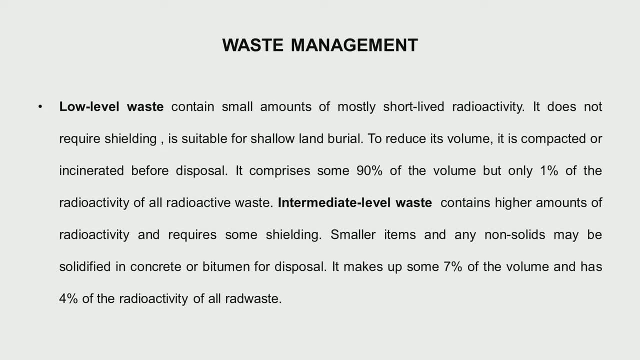 intermediate waste. Then, coming to the intermediate level waste, it will be higher. surely It requires shielding. You cannot do without shielding. Then it makes up about 7% of the volume and has about 4% of the radioactive waste is again in this. 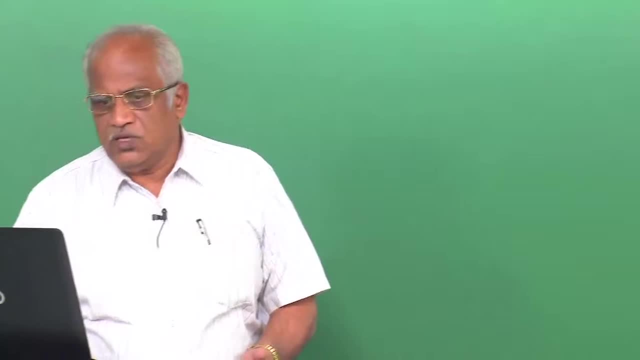 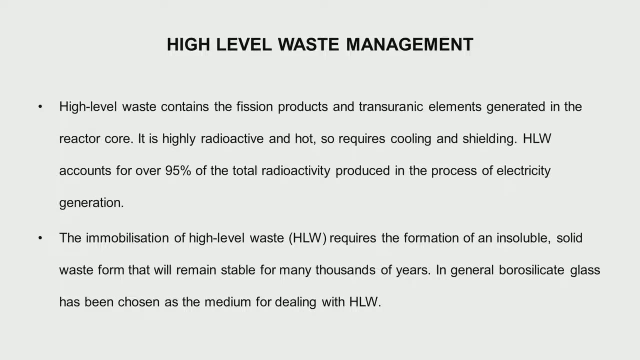 So this again has to be dealt with, again stored for some time. Then the high-level waste, about which you have to be really worried. it is highly radioactive, As I mentioned, it requires cooling and lot of amount of shielding also, and it contains. 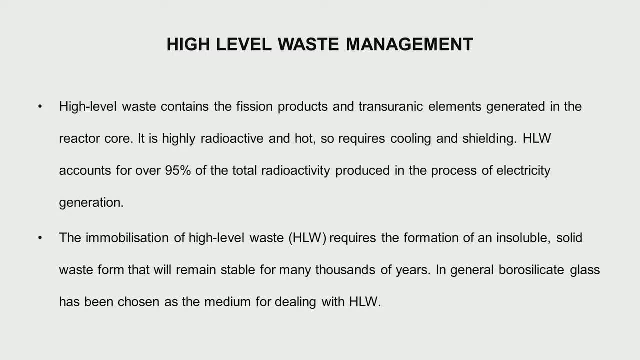 about 95% of the radioactivity, So this waste is the one which we need to be concerned about. So what we do, We have to immobilize the wastes, that is, we have to see that the waste is not able to move. 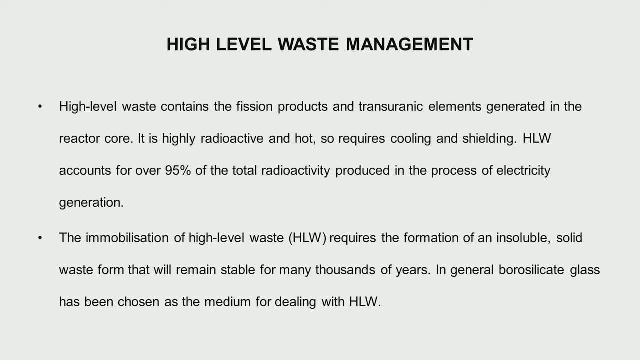 So how to make it immobile? Put it in some other material matrix in which it can get bonded and it does not move. and that is where we find this borosilicate glass has been very good. It is very good as a medium, and borosilicate glass mixed with the fuel is able to hold. 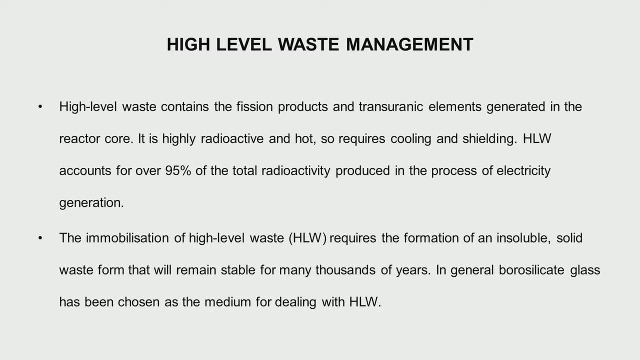 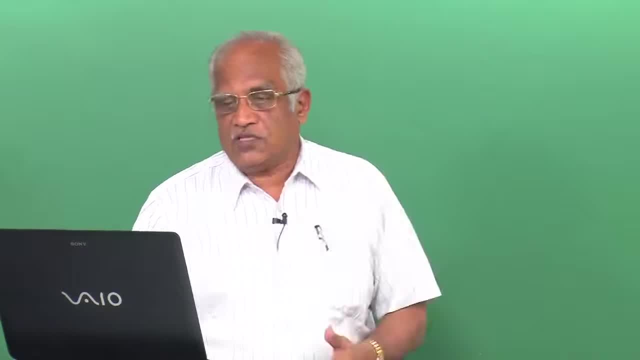 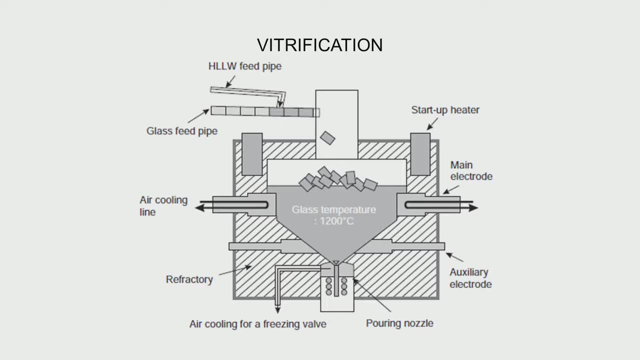 the high-level waste fuel very well bonded, very well, So this is remains stable for a very, very long time because they contain some of the long-lived waste. This is just to give a figure of the process. This process is called vitrification. 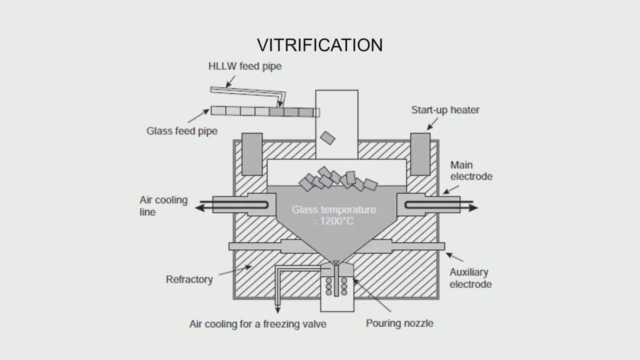 That is, mixing glass and the fuel- high-level waste- And then trying to make this thing. So the glass is molten at about 1200 degree centigrade and we add the waste- high-level waste- and then we pour it and then make it into a solid form, and this solid form we put. 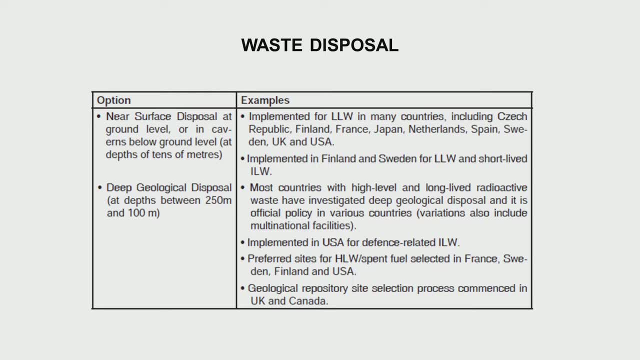 in radiation-shielded casks and put it under the ground. Now, coming to the waste disposal. Okay, So there are different types, as one is near-surface disposal and, as I mentioned, this is done for low-level waste in all countries. it has been done. 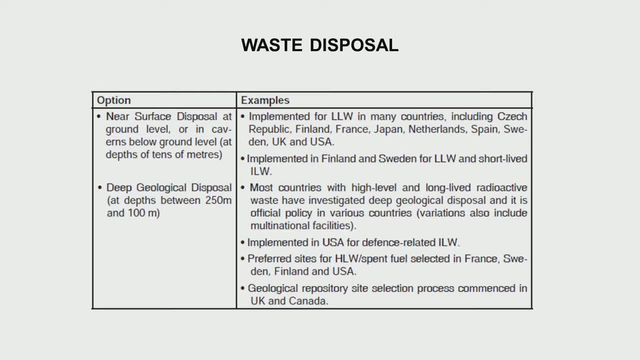 Then deep geological disposal. we are looking for basically for the high-level waste, because they are going to remain for a very long time. So we are looking at what you call geological areas where we are looking for high-level waste. Okay, So the sites are such that they are not going to be approachable for a very long time. 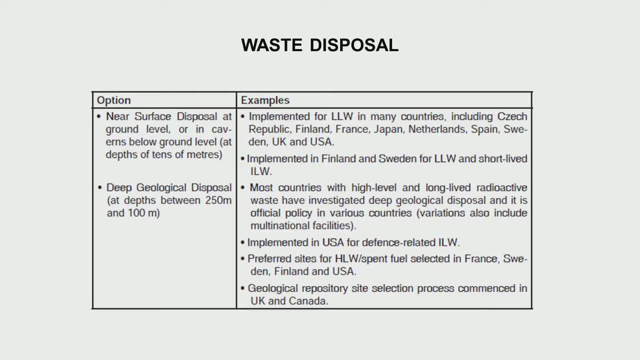 In the USA. the Yucca mountain was the place chosen for putting these high-level waste casks, but they have been delaying due to so many reasons. In fact, because of that, the high-level waste are lying in the plants and it is not a good. 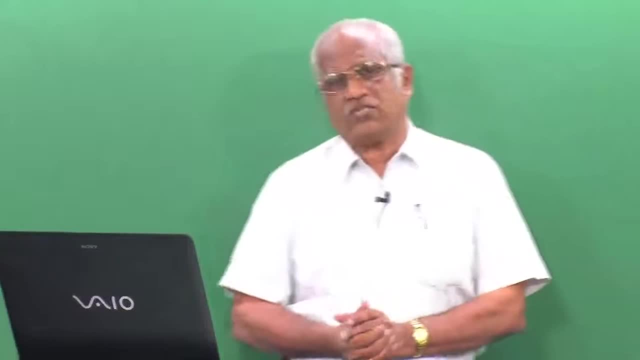 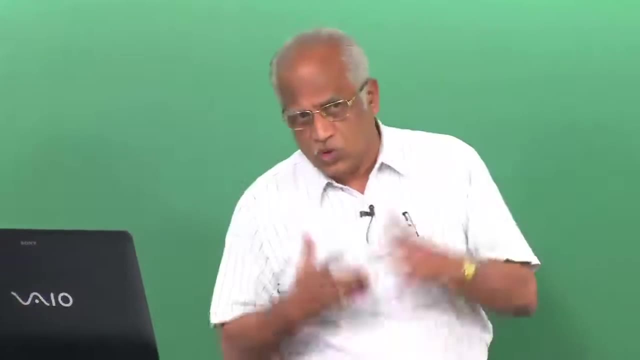 thing. In our own country, we have looked at some geological repositories where the Kohler gold fields were there. Now, practically it is all. there is a lot of place available where, so this is one of the areas which we think could be utilized. 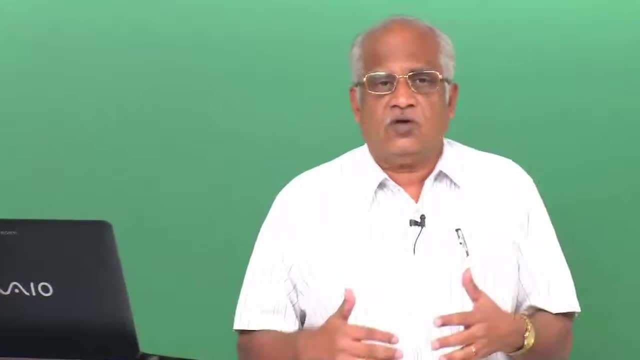 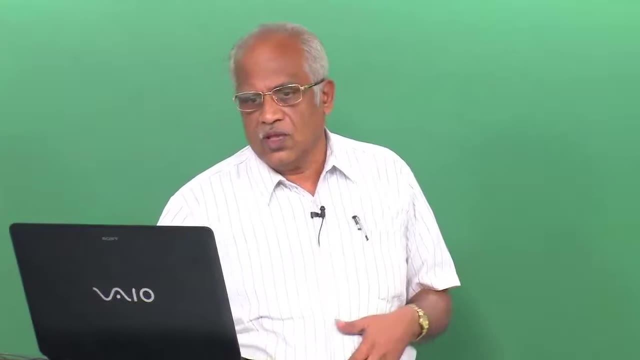 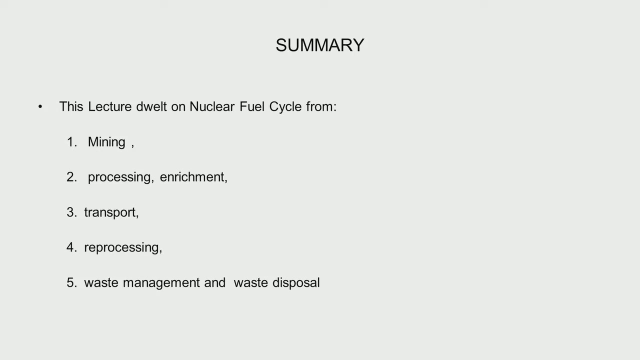 But till now, even though our power program is not very big now, it has not come to a level where have to be there need to be a concern. In brief, Okay, So I can say that this part of the lecture we covered mining. 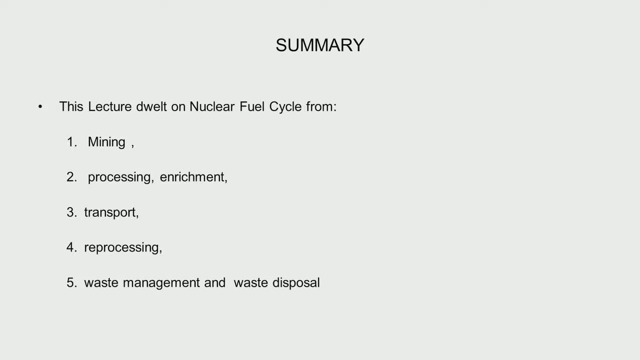 We covered about the processing of the ore, Then the enrichment into of uranium-235 using the centrifuge and the diffusion process. We also had a look at the transportation aspect- That we need to transport things properly in a radiation-shielded casks so that it does. 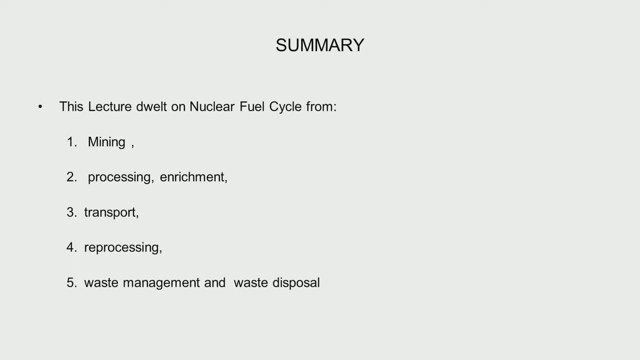 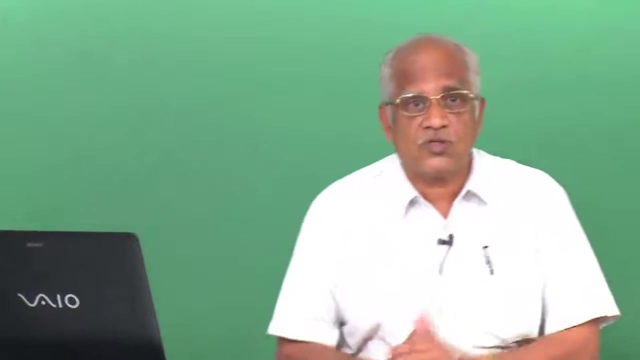 not affect. So at the mining level also we need to be safe Processing everywhere, Every step. we need to be safe reprocessing. It is quite a bit of higher activity wherein we have to be very careful. We deal with solutions also. 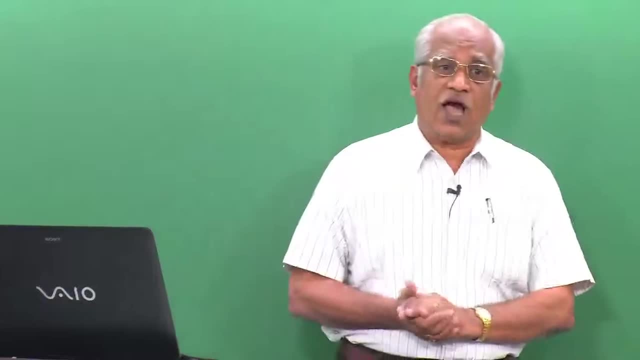 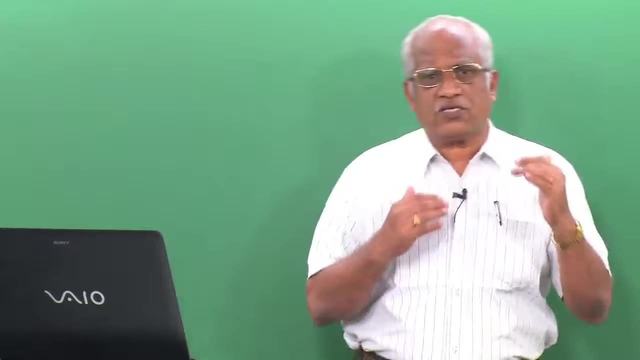 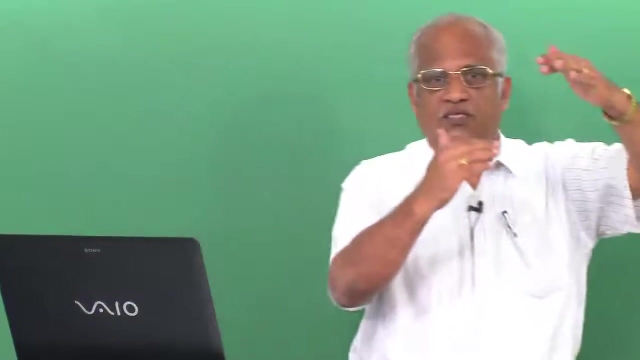 Then, finally, the waste management, Wherein high-level waste, Wherein high-level waste is involved, and the waste disposal. So this lecture, practically I have taken you through the different stages of how the fuel, from its insert, from its birth to its- I should not say- death and its reuse. 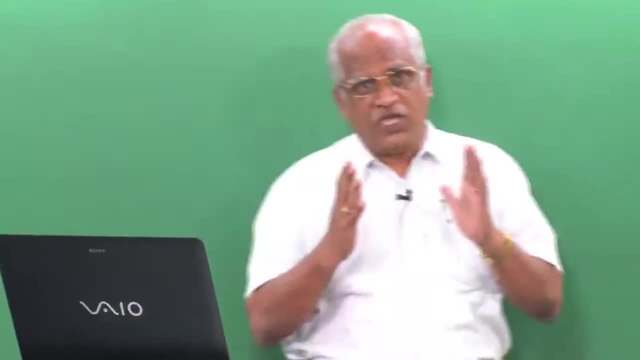 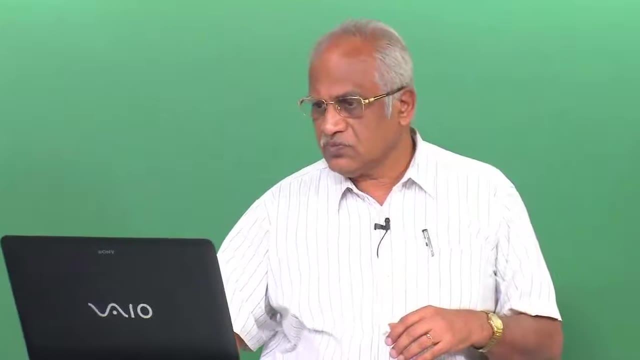 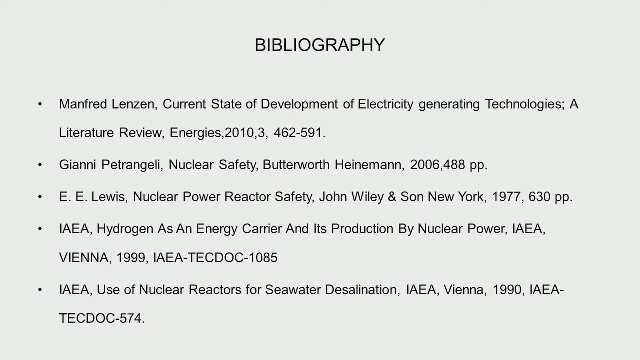 So this gives an idea about the thing. So safety is involved at each and every step of this fuel cycle. Okay, Okay, Thank you. Many of you might be interested to read through some of the literature, So I have just given the bibliography related to my these first two lectures, and there are: 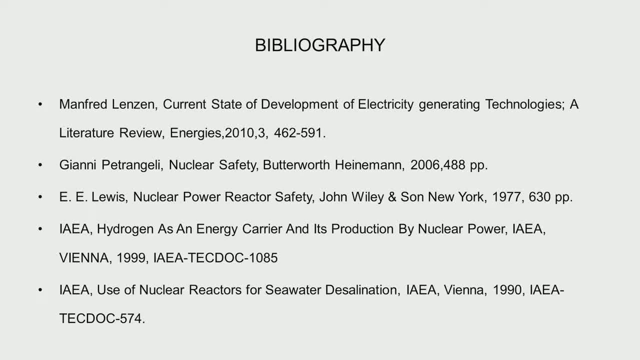 books, many of them published by IAEA, on seawater desalination, hydrogen production. Okay, Okay, It is not only in the publishers. I have read it many times. It is not only in the publishers, It is in the New York Times.